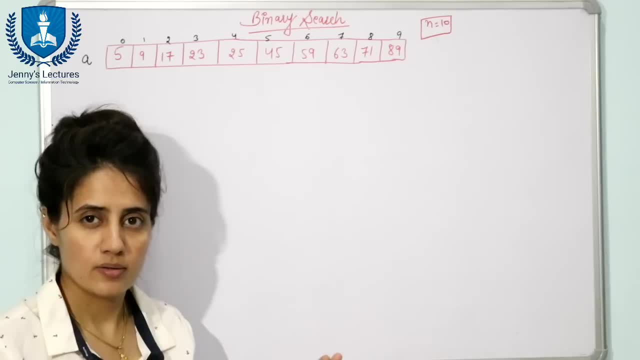 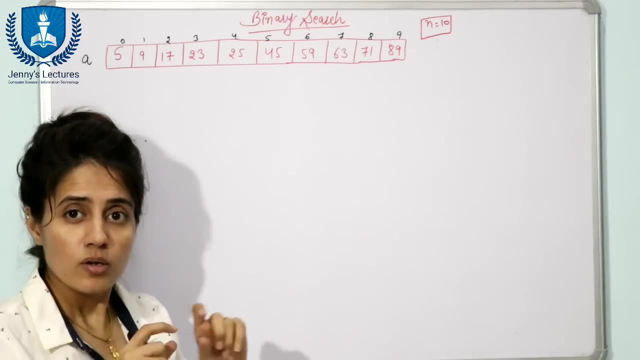 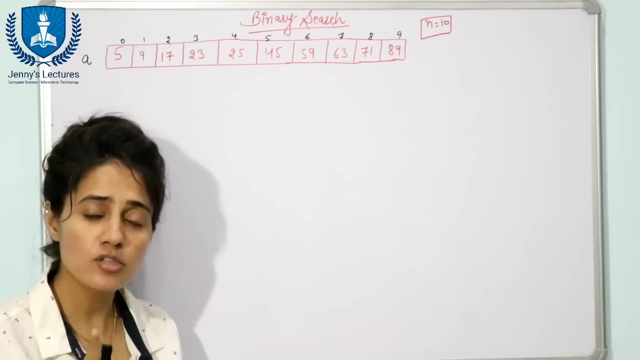 algorithm is what the array should be sorted. See here you can see I have taken this example. but the data in this array is what sorted? right? If the data is not sorted, then you cannot apply binary search on that array. You have to first sort the array, then you can apply binary search for searching. 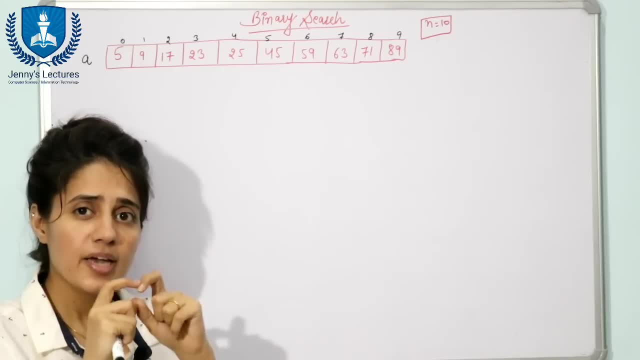 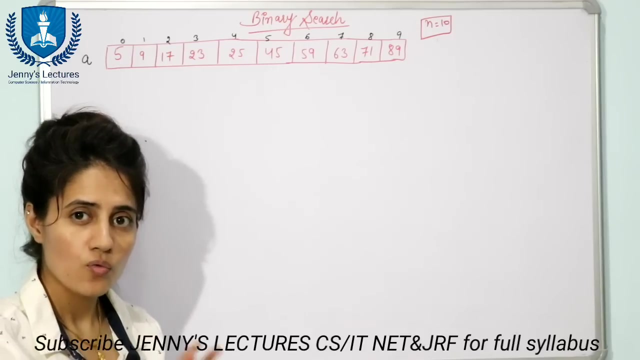 So here the precondition for this binary search is the array should be sorted. That is not a case in linear search. That linear search works fine on the sorted array as well as on unsorted array. Now we will see how this binary search algorithm will work. Fine, see. So now we are going to search. 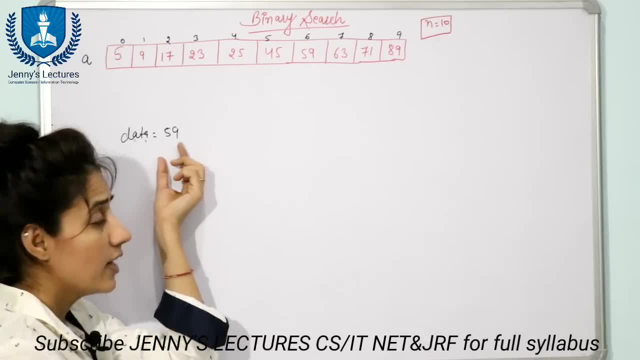 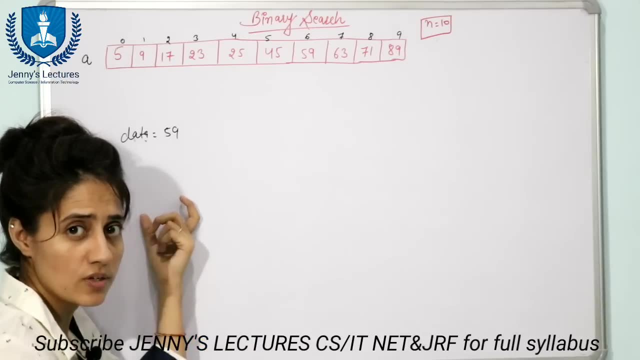 for the data, or you can say key 59. Is this 59 present in this array or not? and if present, your code should return where this 59 is present: The index at which this 59 is present, See. one more important point about this binary search algorithm is what it is: divide and conquer technique. 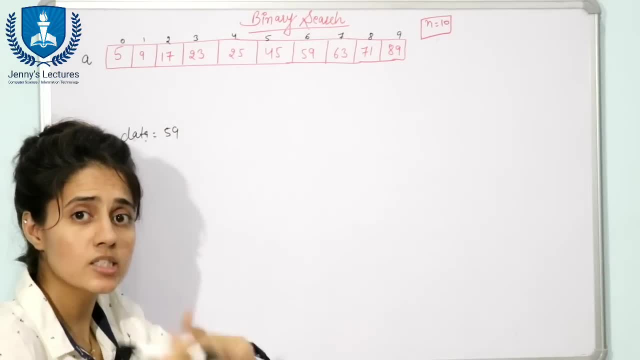 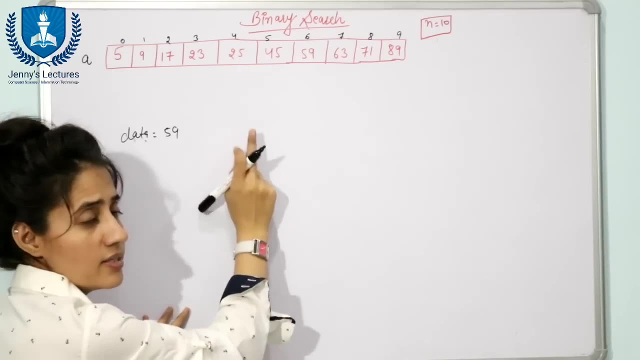 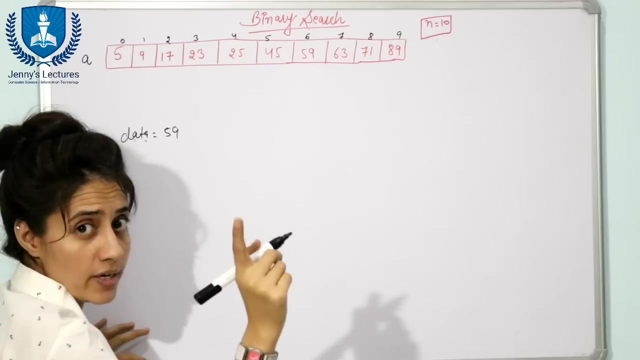 It means it is going to divide the array into two halves, Recursively divide the array. Now, how recursively it will divide the array into sub arrays. we are going to see, See. in this case, we are going to find out the middle element of the array. Fine, So we are going to take two variables. First, 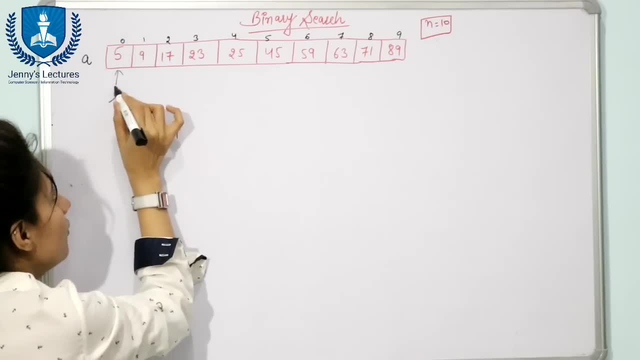 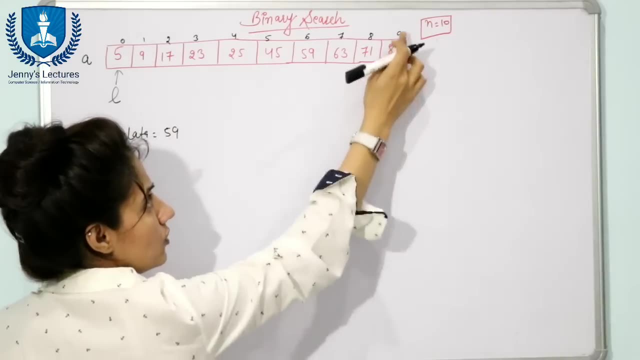 is here left variable, and we are going to point left here Means l value is 0.. Next variable is right and the value of this right is 9, or you can say n minus 1.. So in this algorithm we are going to find out the. 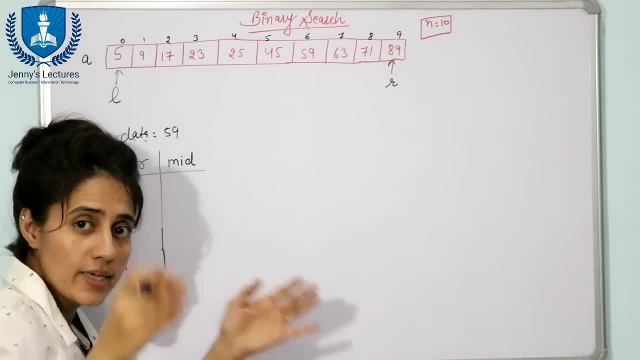 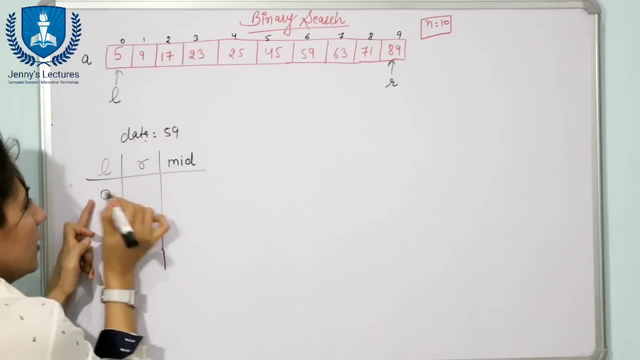 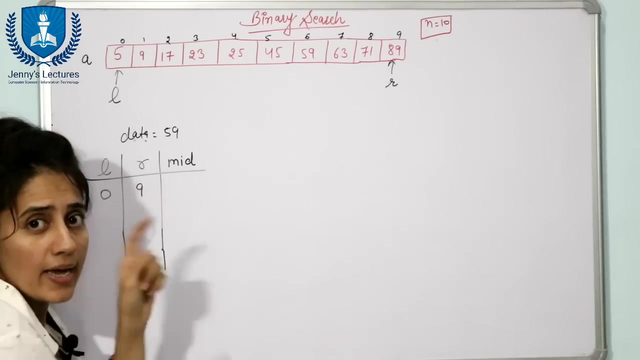 mid position of the array, from where we are going to divide the array into two halves. Fine, See, first of all, the left is 0 and the right is 9 in this case. Now find out the mid of this one. How to find out mid? l plus r divide by 2.. l plus r divide by 2 and we are going to take the floor. 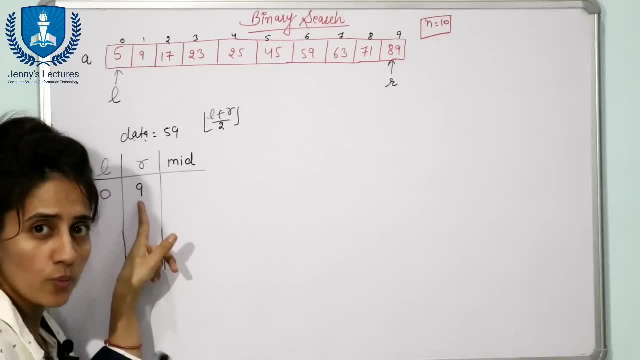 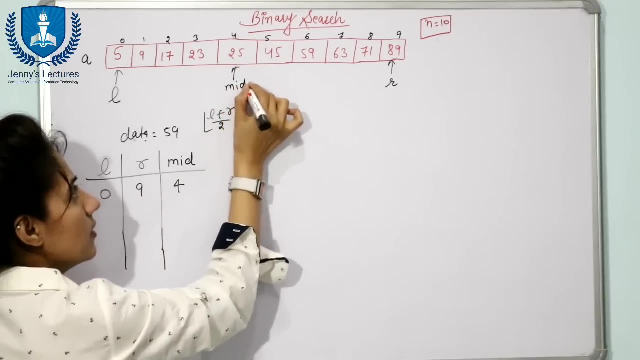 value of this one, 0 plus 9, divide by 2, is what 4.5 floor value is 4.. So mid is what 4.. So at index 4 we are having mid. now Now here three cases can be there. First case is the data. 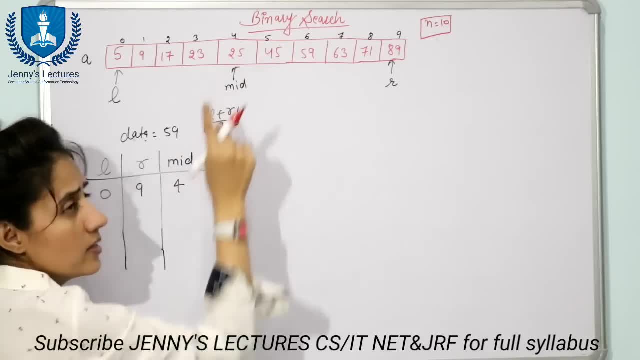 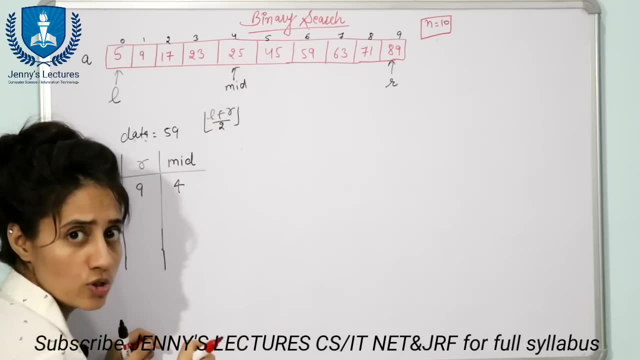 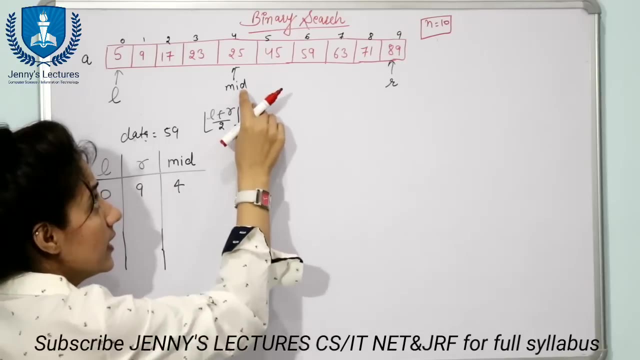 you want to find out is equal to the data at the mid position. Fine. Second case is the data is less than the data which is at mid position. or, third case, is the data you want to find out- the key you want to find out, find out- is greater than the data which is at mid position. So, 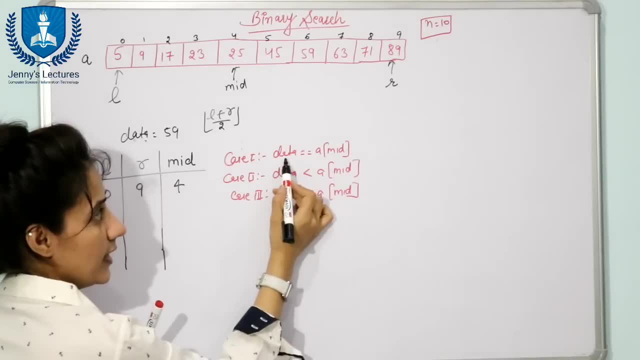 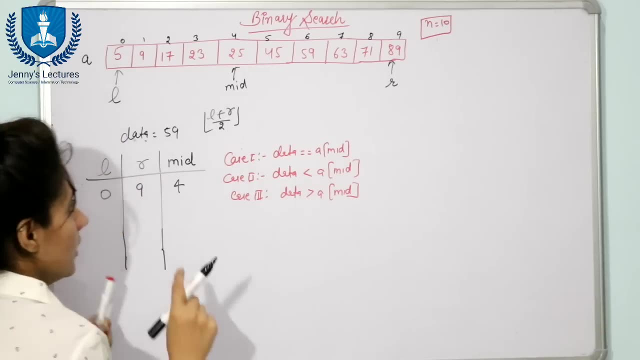 these are three cases. Fine. Data is equal to this mid, Data is less than this, a of mid and data is greater than a of mid. Three cases can be there Now. see here: the data is 59 and mid is 4.. 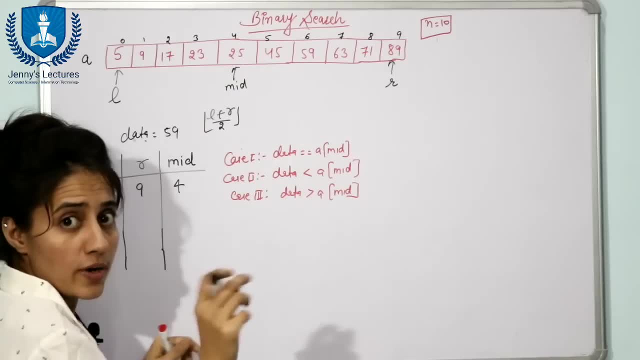 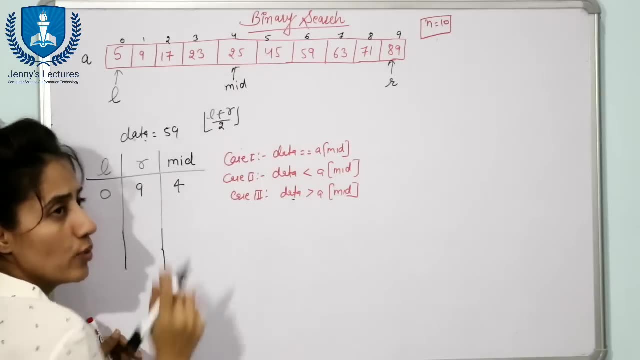 Now, what is that? a of 4? a of 4, the data is 25.. So here the case is this one: The data is 59, and 59 is greater than a of mid. a of mid is 25.. Right, So now we can say that the data is greater than. 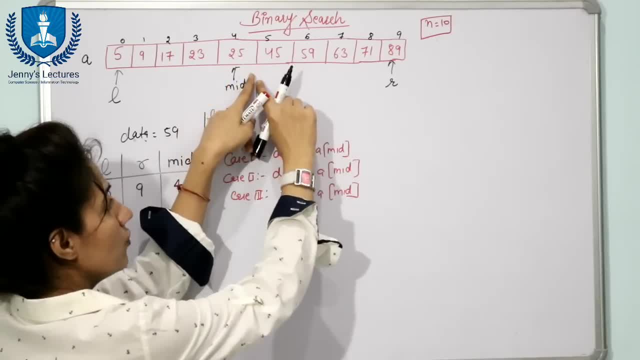 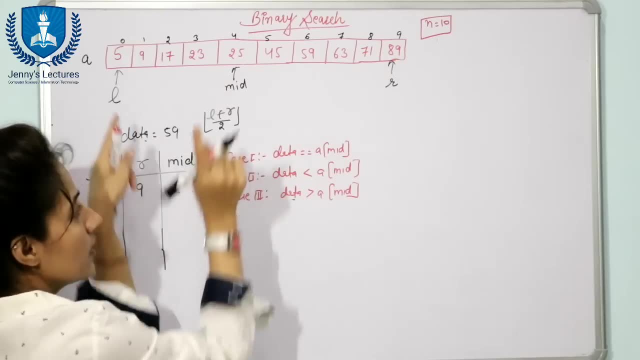 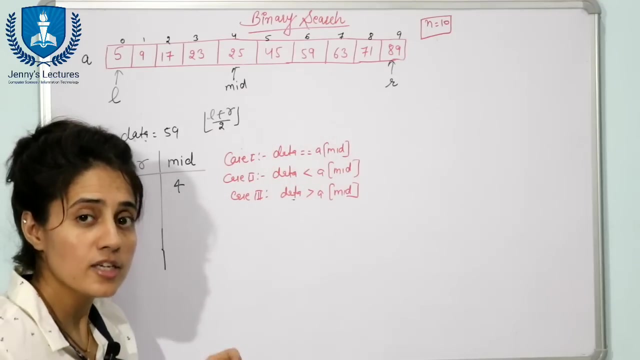 that this data is present to the right of this mid. in this subarray, in this subarray. Now, we have divided this array into two parts. One is this one and one is this one. Now we can say this 59 is present to the right of this mid. Now, how you can say this? because we know that the array is sorted. 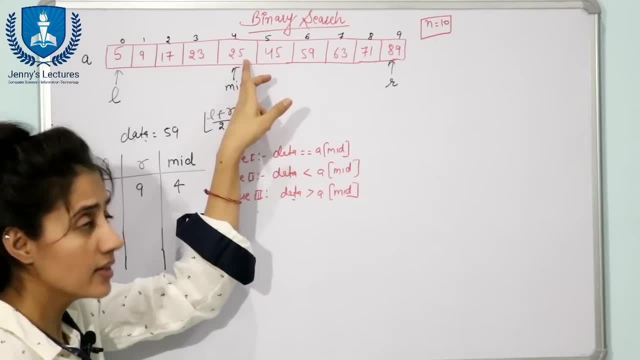 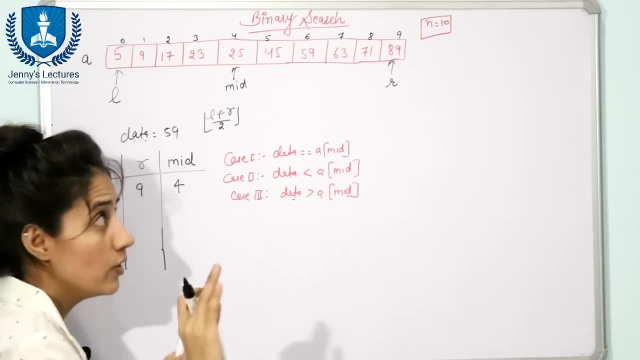 and if array is sorted, then all the data which is greater than 25 must be present to the right of this 25.. Right Now we are going to see, we are now we are going to search only in this array. We have divided our 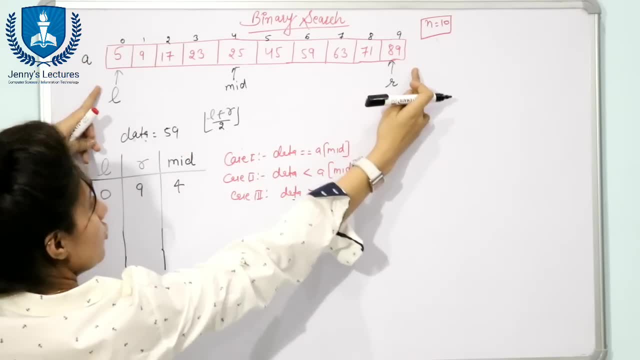 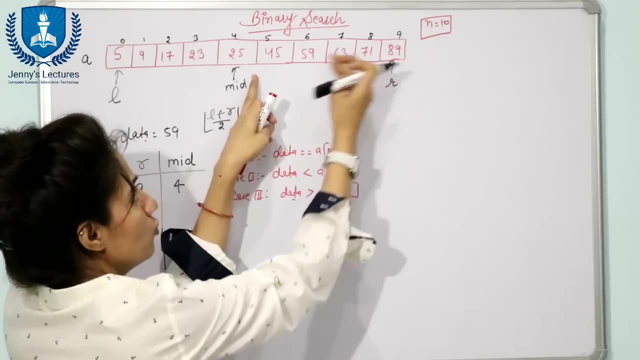 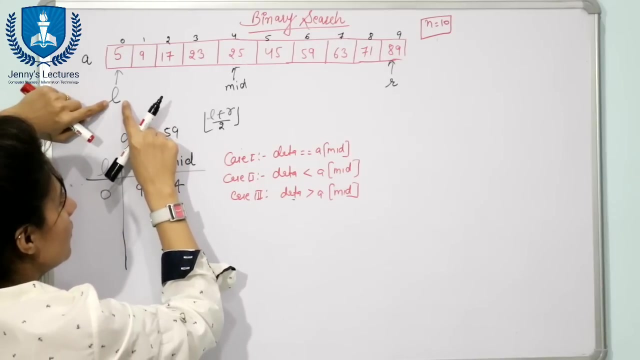 search space. First, at first, our search space is this one. After first comparison, we have divided it into half. Now this is our search space. We are going to search from here to here now, Fine, So if this is the case, then this left, then this left variable should be moved here only to the 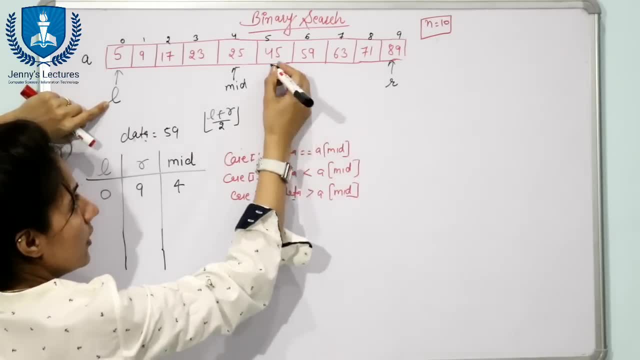 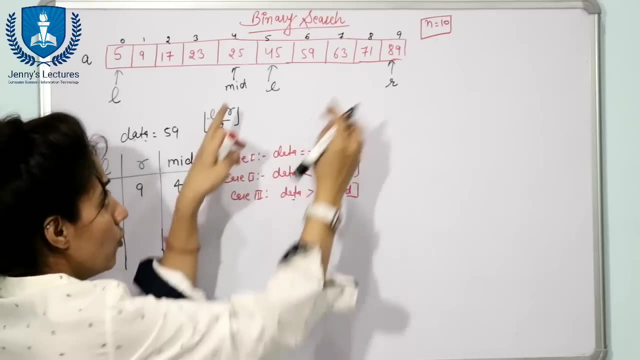 right here, Right Right, This side towards the right. So now, here we have our left. Our left now becomes mid plus 1, because we are going to work only in this array now and r is as it is, that is 9.. Again, repeat the. 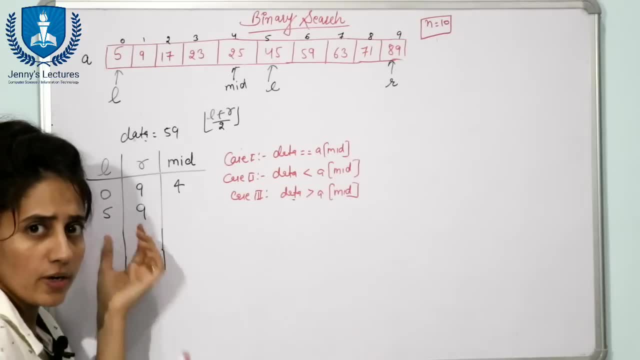 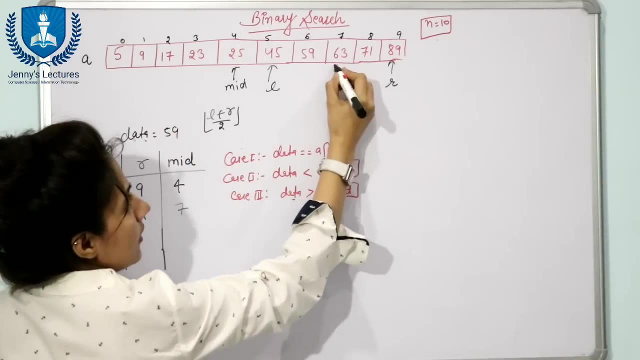 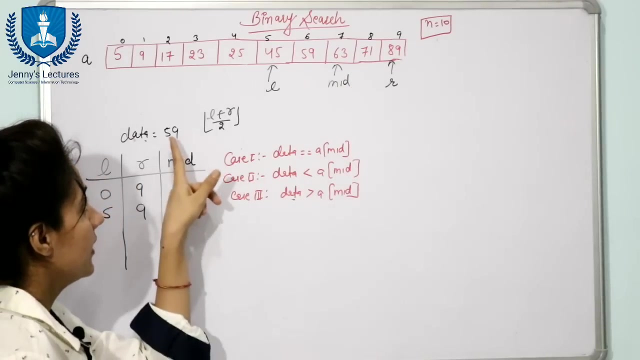 same step. Find out: mid 5 plus 9.. 14 divide by 2 is 7.. Mid is what 7.. Now, mid is what Here? 7.. Now again, three cases can be there. Now check Data is 59.. Is 63 same as 59?? No, Now the case is here. 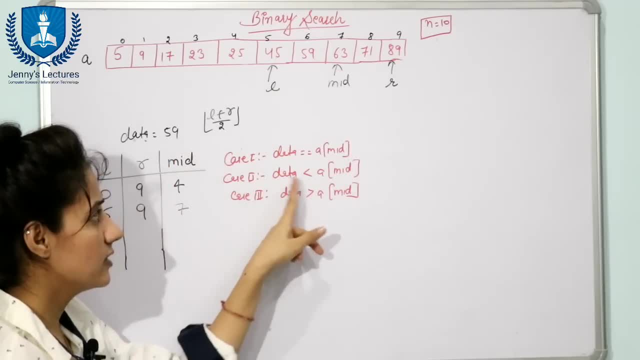 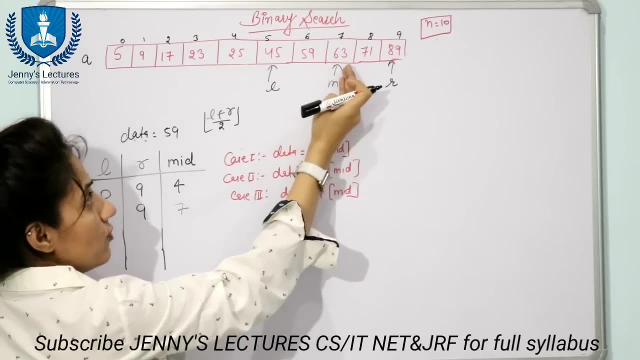 59 is the data is less than 63.. This second case: Data is less than a of mid. Now what you can say? data is present to the left of 63 here only because data is less than 63 and array is sorted. So now, 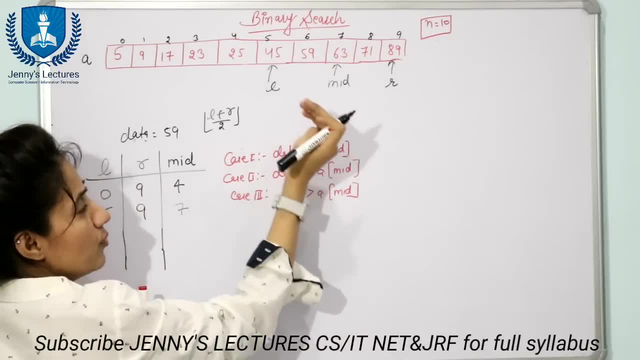 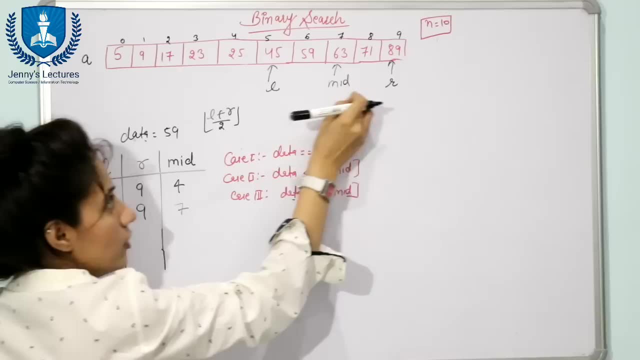 so now, if data is present to the left of 63, here, only because data is less than 63 and array is sorted. So now, if data is present to the left of mid, to the left of mid, in that case what you will do, Left would be, as it is, 5 and this right would be moved towards this side. So now right becomes. 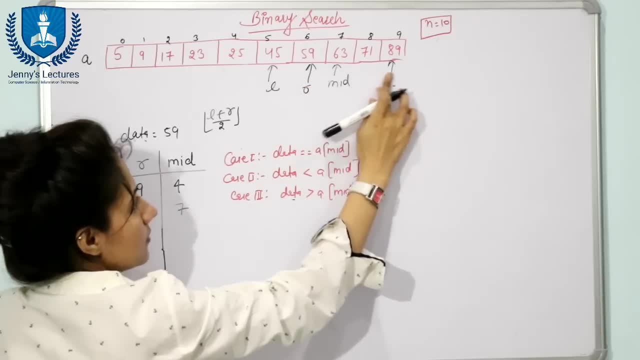 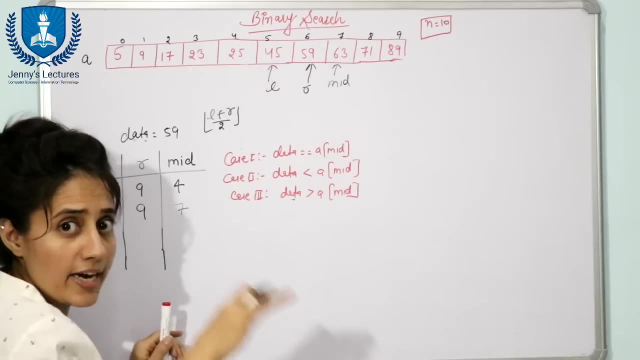 mid minus 1.. Now here we have right, because now we are going to work only in this space, here only. We again divided the array into two parts. That is why I was saying we recursively divide the array into two parts. Fine, until you find the element. 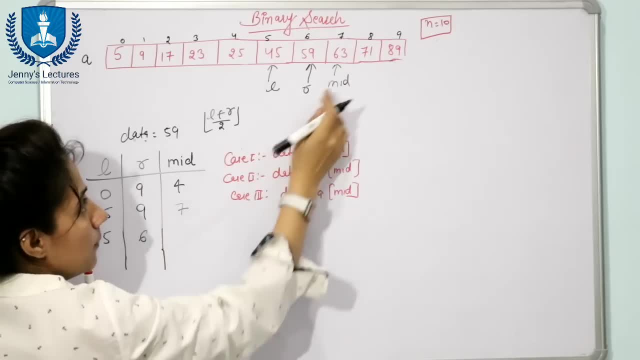 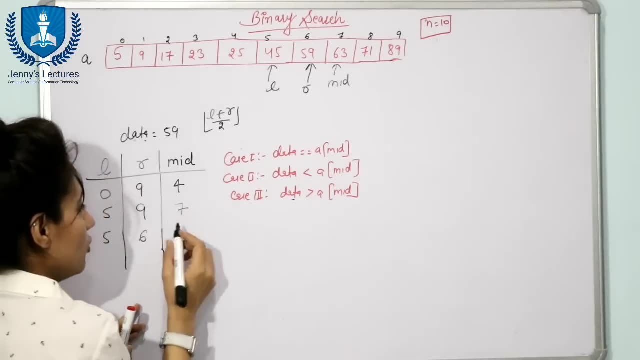 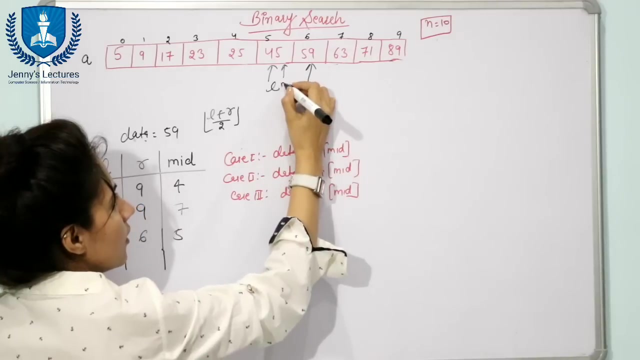 So now R is what? 6.. Mid minus 1.. 7 minus 1 is 6.. Now again find out: the mid: 5 plus 6 is 11 by 2.. That is 5.5.. Floor value is 5.. So mid is now here, 5.. L is also 5 and mid is also 5 now. 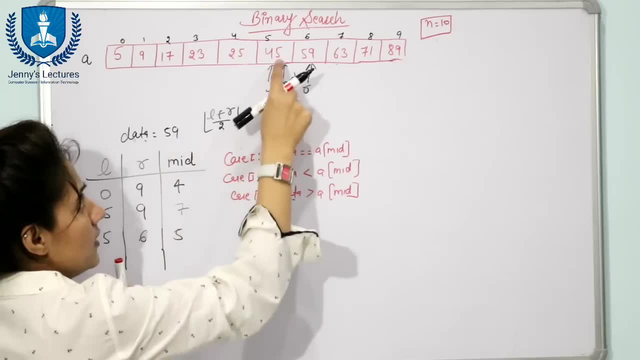 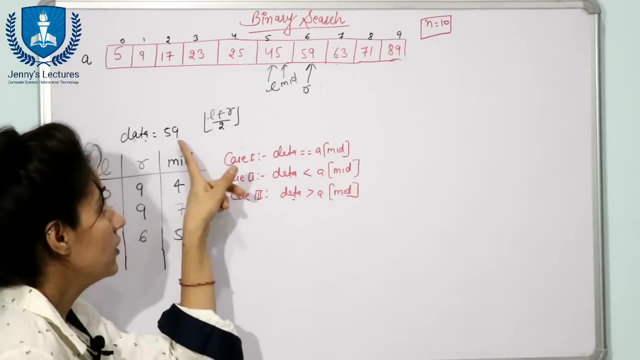 Right Now check: Is 59 same as a of mid? No, 59 is greater than a of mid. It means 59 is present to the right of mid, To the right array of this mid Right. And if this, this is: 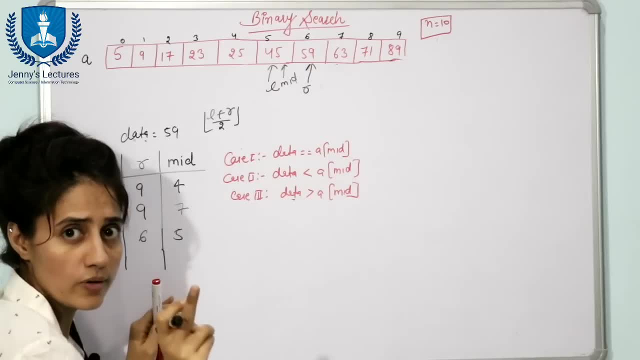 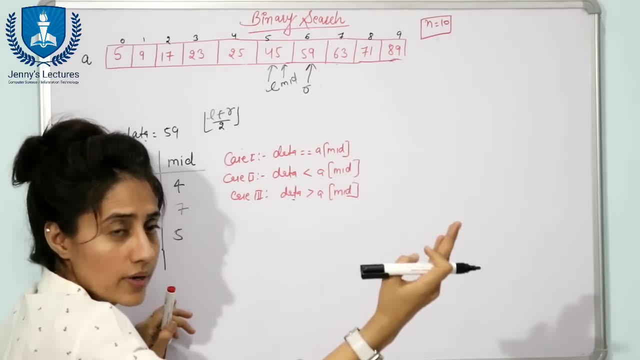 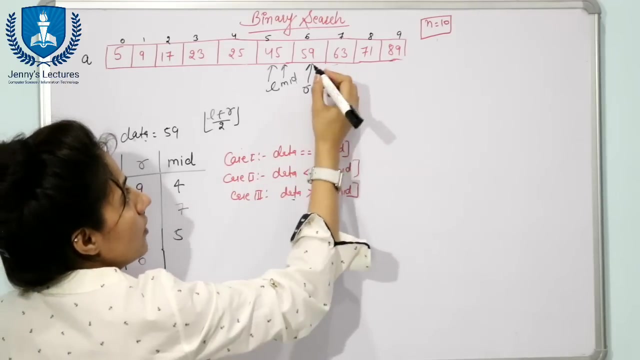 present. the data is present to the right of the mid. in that case, what? what we will do? We will move left towards this side Means: left becomes mid plus 1, now Right. So left becomes mid plus 1.. That is, 5 plus 1 is 6.. Right remains as it is. So now, now, here we have left and here we have. 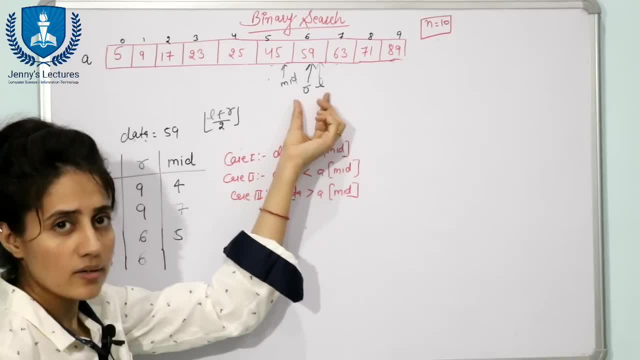 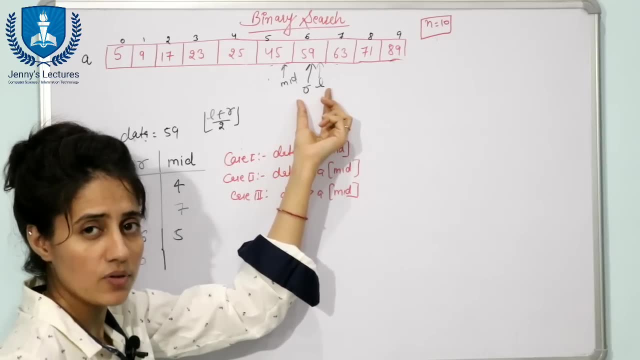 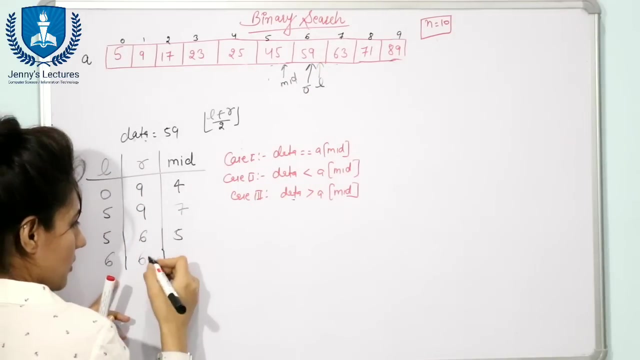 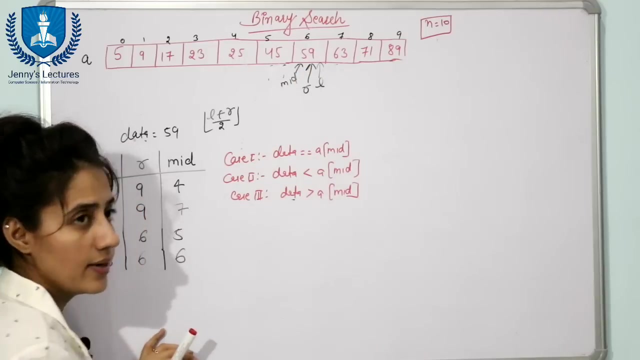 right. only Left and right are at pointing at same index. It means in this we have only one element In the array. we have now only one element, So now we have only 59. See Again. find out: middle 6 plus 6 is and divide by 2 is 6.. Now mid is also here At 6.. Now check If data is equal to is. 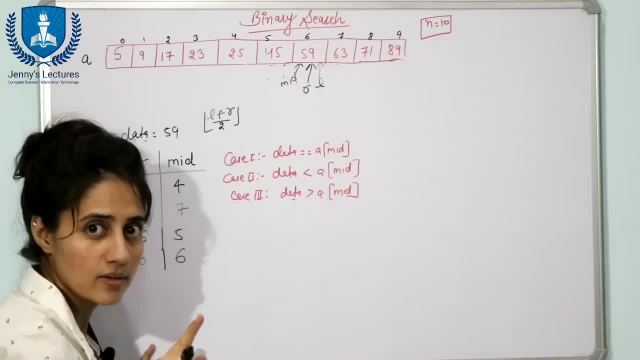 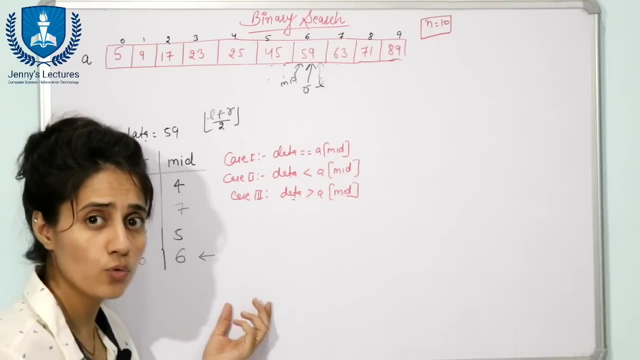 equal to a of mid. 59 is equal to a of mid. Yes, Now, this is the stopping condition. We found the data. So now, here you are going to stop And you are. you are going to return mid. Return mid means you are going to return the index 6, where the data is present. Fine, 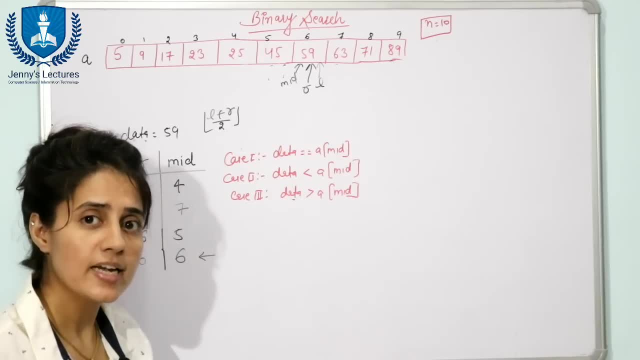 So this is the one stopping condition. Now, second case is if data is not present in the array. In that case, when you are going to stop your searching algorithm, Let us take that case only. That case also: Is 25 equal to 59?. 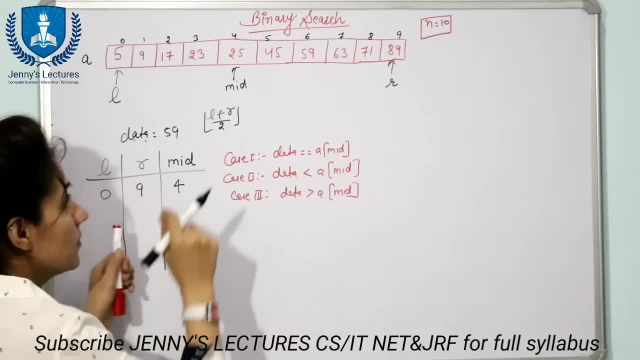 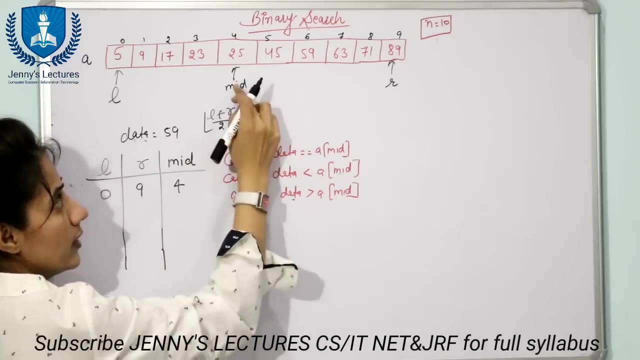 Is this you want to search? No, So second case is this data. This data is what? This data is greater than the data which is at mid position. So here the case is this one: The data is 59, and 59 is greater than a of mid. a of mid is 25.. Right, So now we can. 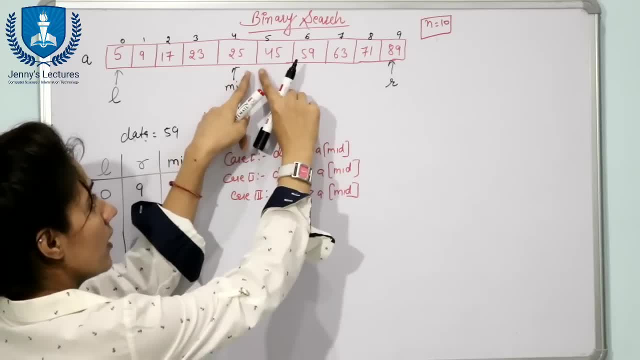 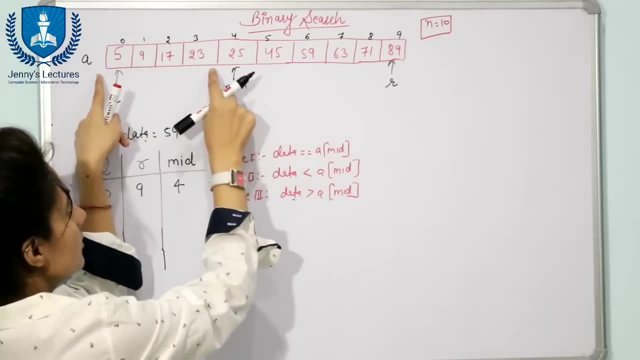 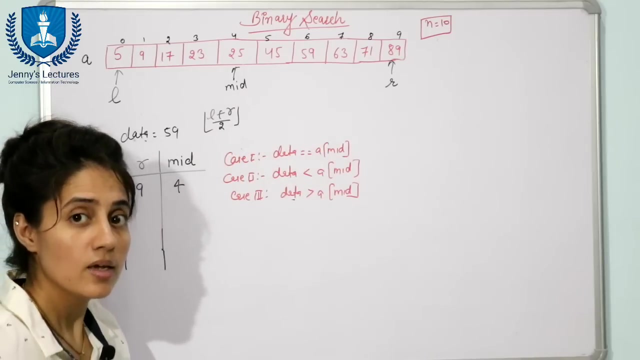 say that this data is present to the right of this mid In this sub array, In this sub array. have divided this array into two parts. one is this one and one is this one. now we can say this 59 is present to the right of this mid. now, how you can say this? because we know that the array is sorted. 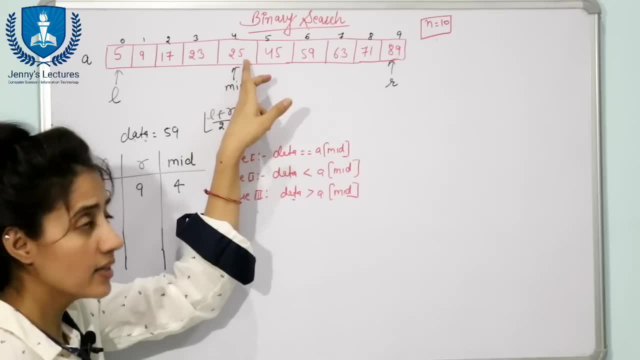 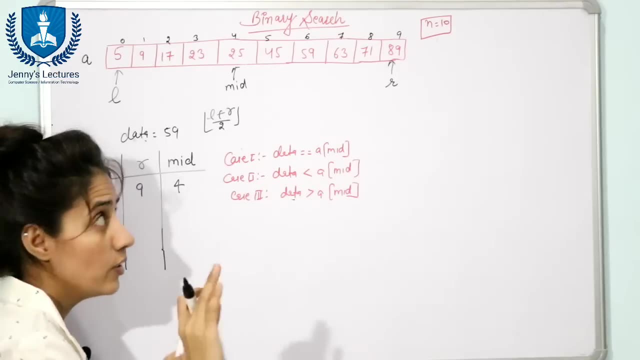 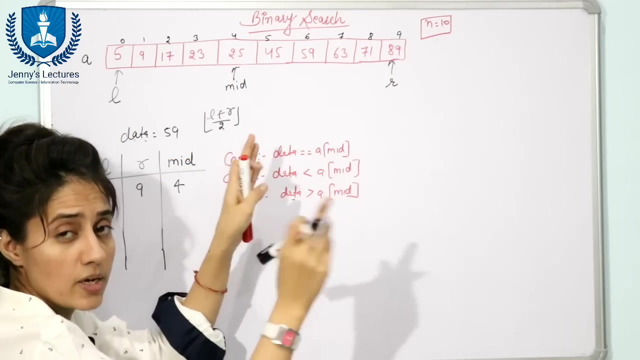 and if array is sorted, then all the data which is greater than 25 must be present to the right of this 25. right now we are going to see we are. now we are going to search only in this array. we have divided our search space first. at first, our search space is this one. 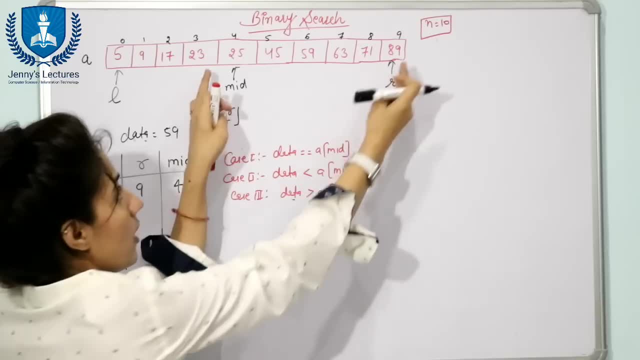 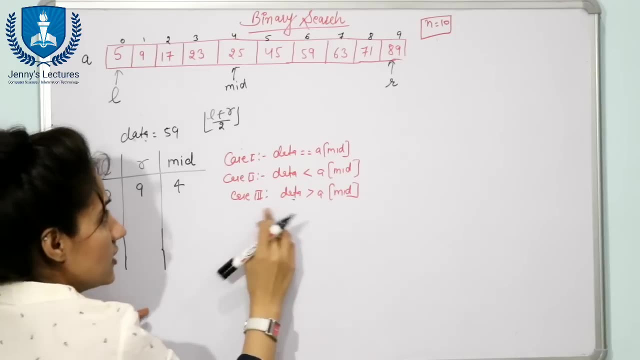 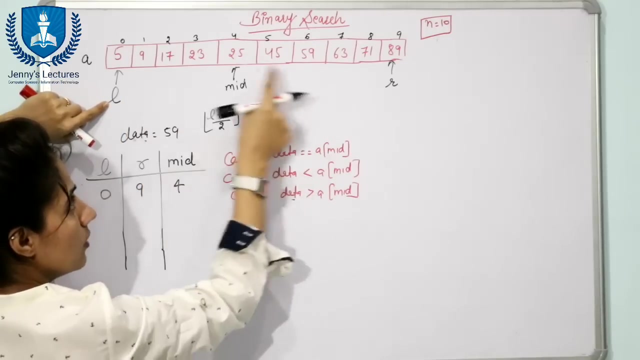 after first comparison, we have divided it into half. now this is our search space. we are going to search from here to here. now, fine, so if this is the case, then this left, then this left variable should be moved here only to the right, here, this side towards the right. so now, here we have our 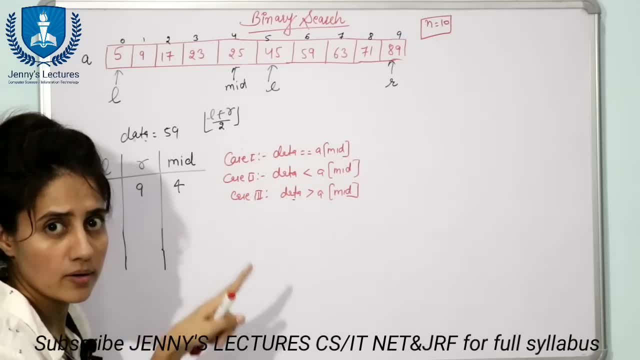 left, left. our left now becomes mid plus 1, because we are going to work only in this area now and r is as it is, that is 9.. again, repeat the same step. find out: mid 5 plus 9, 14 divided by 2 is 7. 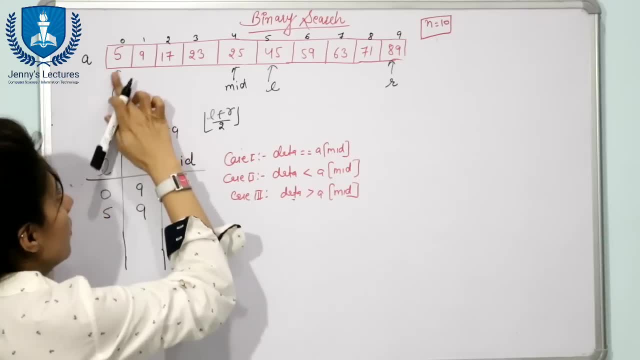 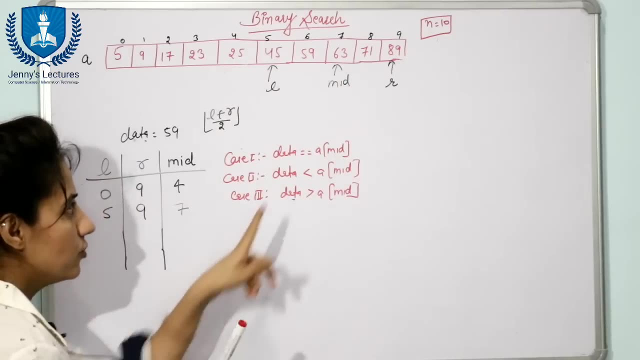 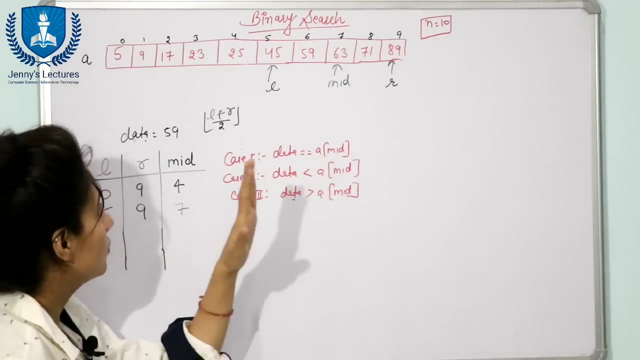 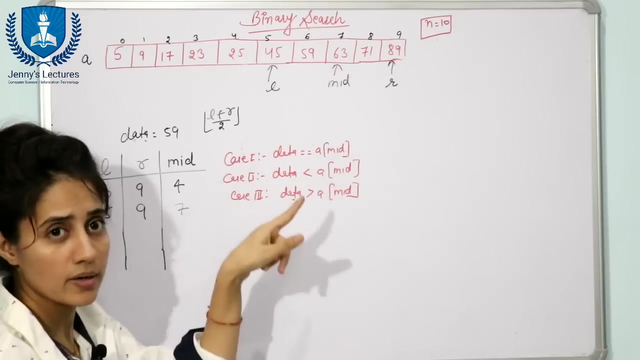 mid is what 7. now. now mid is what here, 7. now again, three cases can be there. now check data: is 59, is 63 same as 59? no, now the case is here: 59 is the data is less than 63. this second case: data is less than a of mid. now what you can say data is. 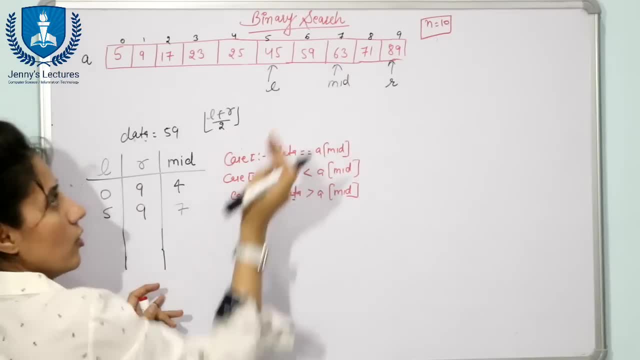 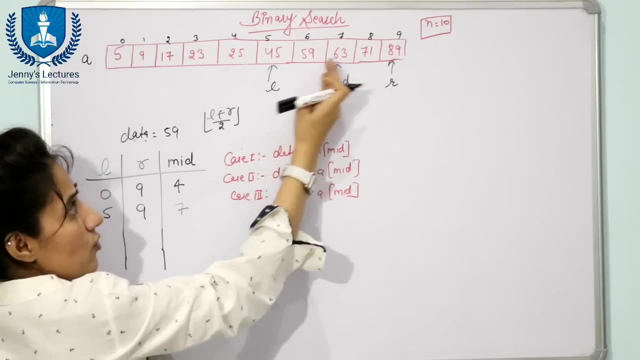 present to the left of 63 here only because data is less than 63 and array is sorted, so now. so now, if data is present to the left of 63 here only because data is less than 63 and array is sorted, then to the left of mid, to the left of mid. in that case, what you will do, left would be as it is. 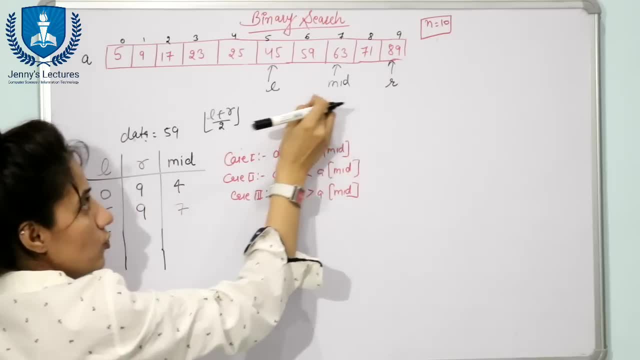 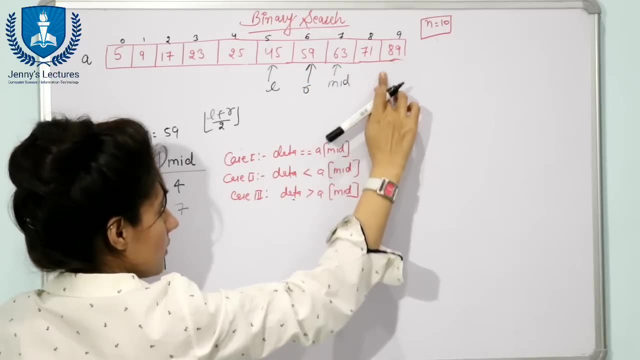 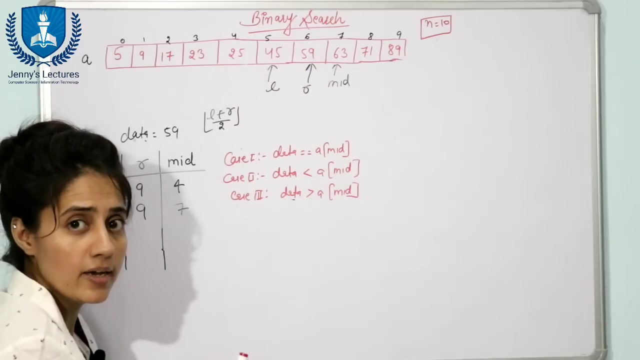 5 and this right would be moved towards this side. so now right becomes mid minus 1. now here we have right, because now we are going to work only in this space, here only. we again divided the array into two parts. that is why i was saying we recursively divide the array into two parts. 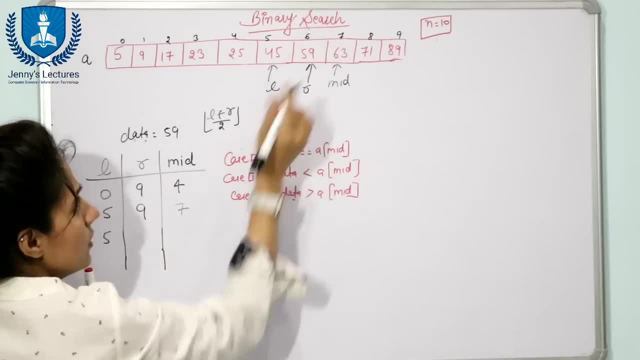 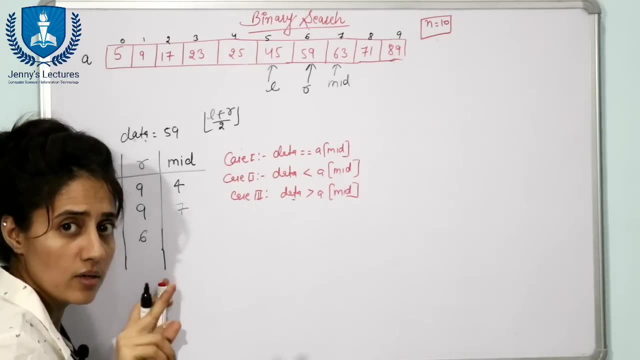 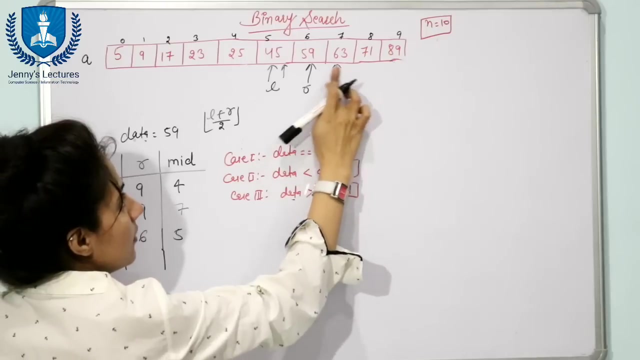 fine, until you find the element. so now, r is what? 6 mid minus 1, 7 minus 1 is 6. now again find out. the mid. 5 plus 6 is 11 by 2, that is 5.5. floor value is 5. so mid is now here 5, l is also 5 and mid is also 5 now. 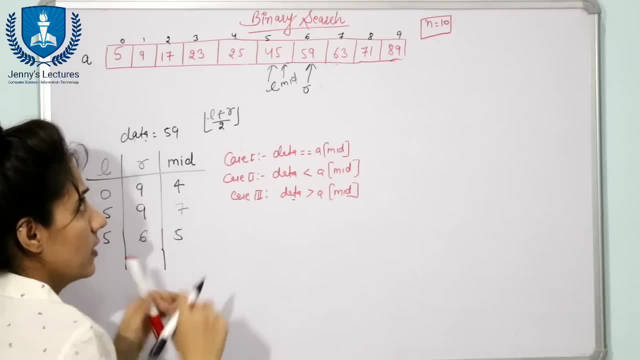 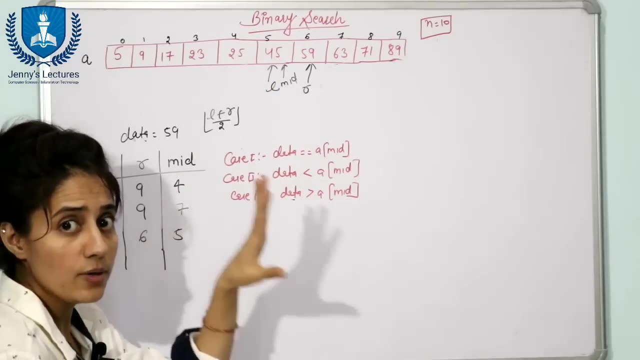 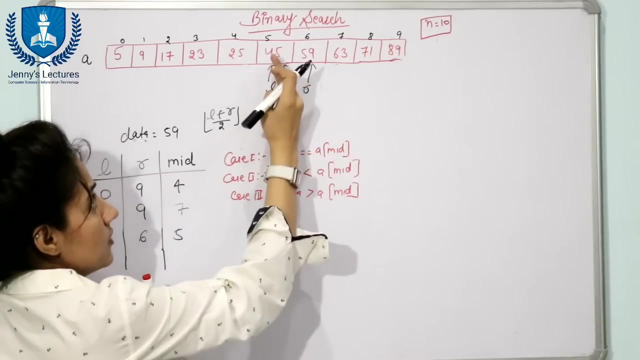 right now. check: is 59 same as a of mid? no, 59 is greater than a of mid. it means 59 is present to the right of mid, to the right area of this mid right, and if this, this is present, the data is present to the right of the mid. in that case, what? what we will do? we will move left. 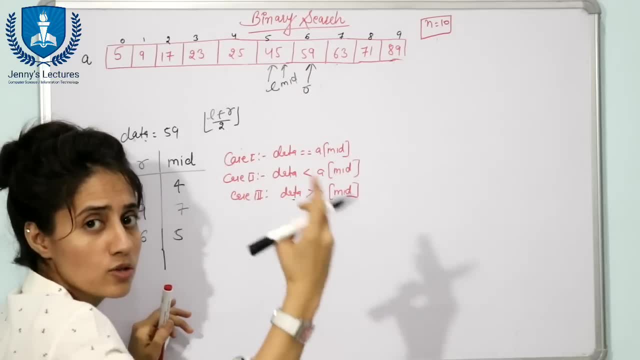 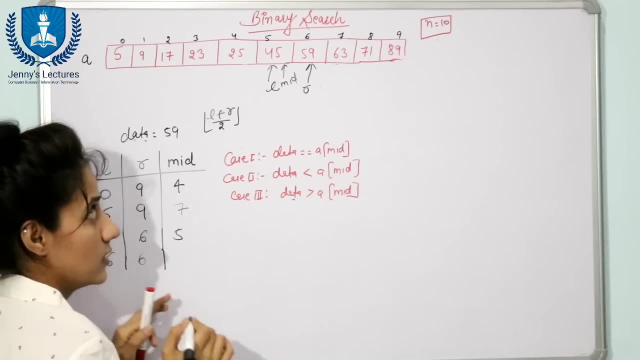 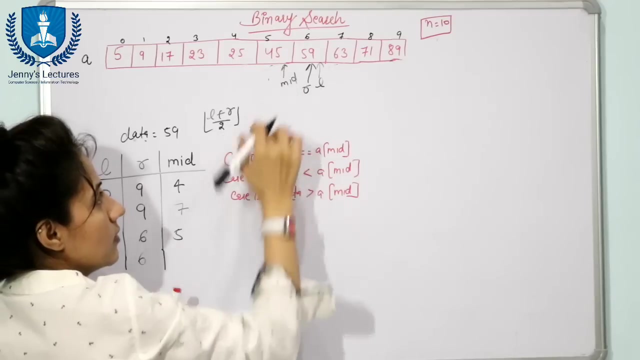 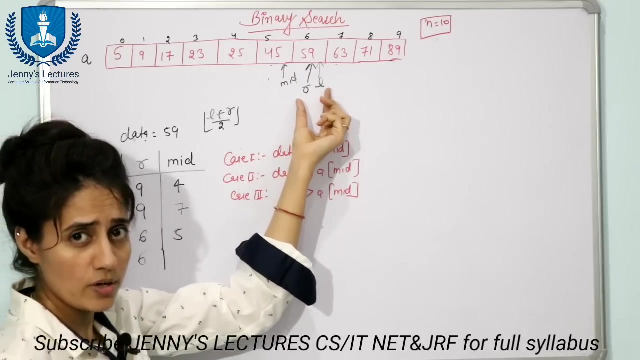 towards this side means left becomes mid plus 1, now right, so left becomes mid plus 1, that is 5 plus 1 is 6. right remains as it is. so now, now here we have left and here we have right, only so if left and right are at pointing at same index. it means in this we have only one element. 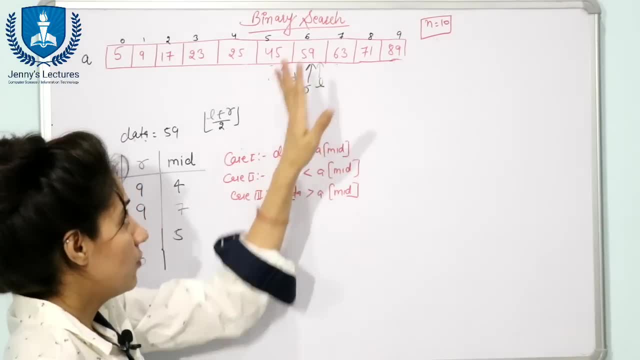 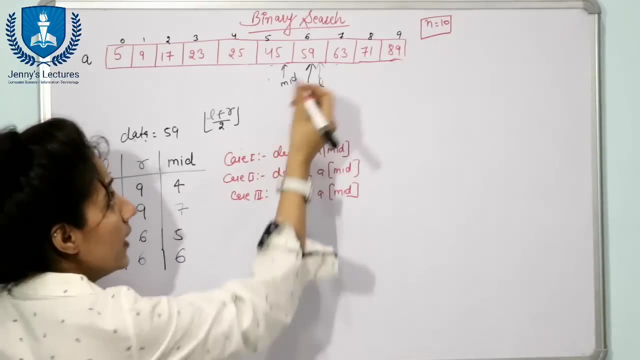 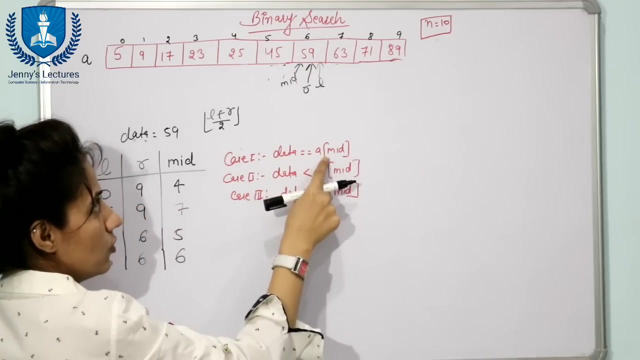 in the array. we have now only one element, so now we have only 59. see, i can find out middle 6 plus 6 and divide by 2 is 6. now mid is also here at 6. now check if data is equal to. is equal to a of mid. 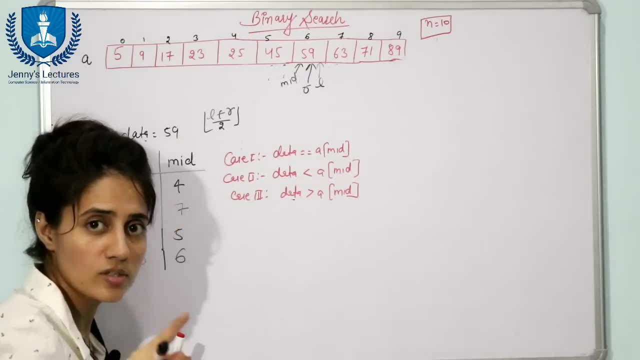 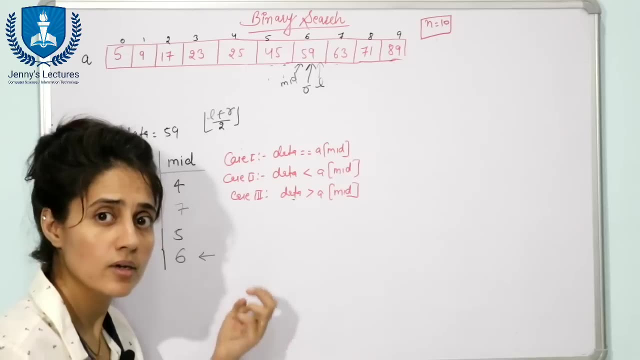 59 is equal to a of mid. yes, now, this is the data of mid. so now we have only one element. so now we have only one element. so this is the stopping condition. we found the data. so now, here you are going to stop, and you are. you are going to return mid. return mid means you are going to return the. 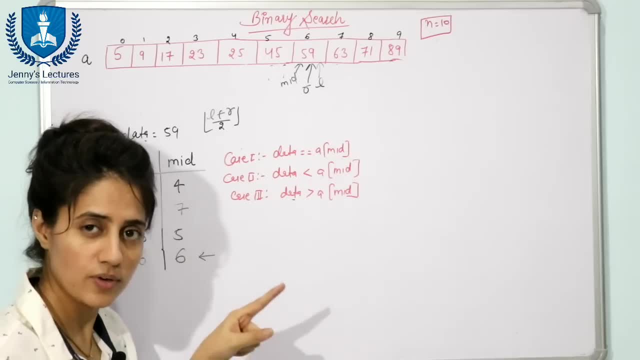 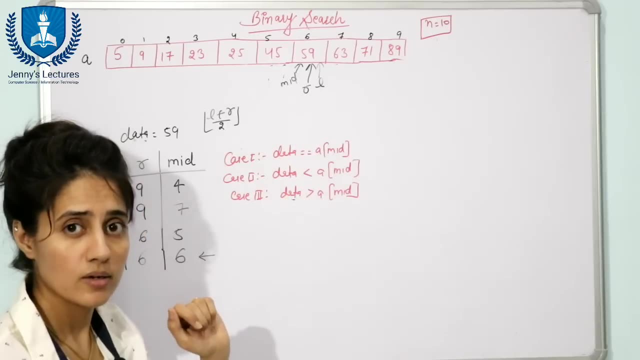 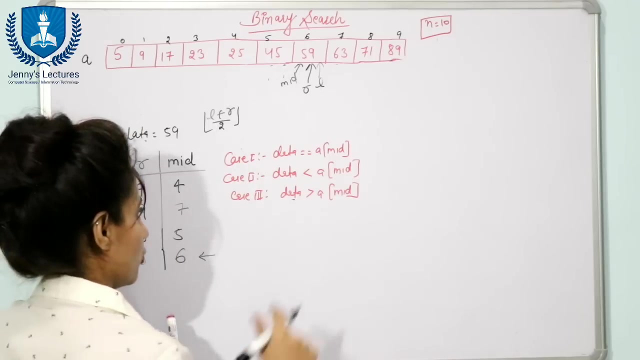 index 6, where the data is present. fine, so this is the one stopping condition. now, second case is if data is not present in the array, in that case, when you are going to stop your searching algorithm, let us take that case, only that case. also now, let us take. you want to find out? 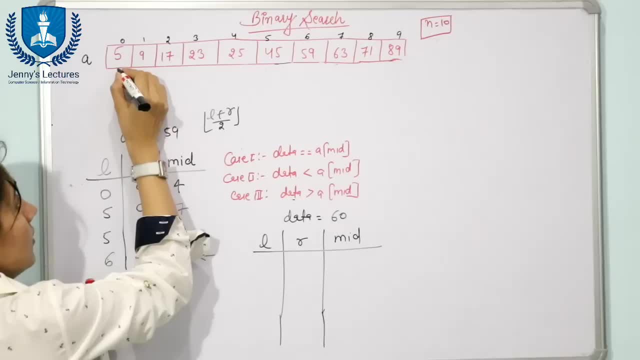 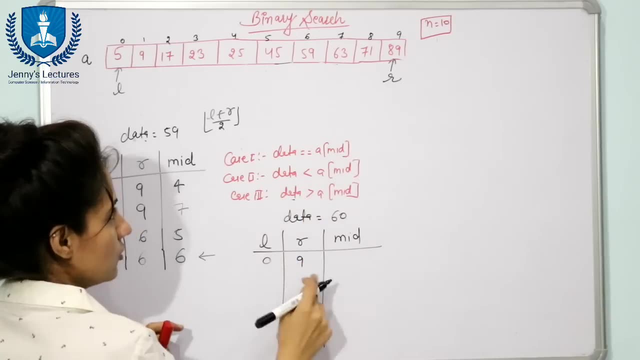 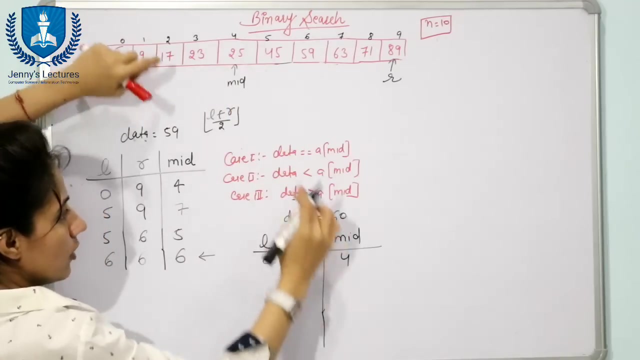 60. see. 60 is not present here now. we will see same. l is here only and right is here only now. left is 0 and right is 9. mid is what? 4 at 4, you have what 25 here we have mid. this is not equal to 60. 60 is greater than this 25. so data is present to the right of 25. if data 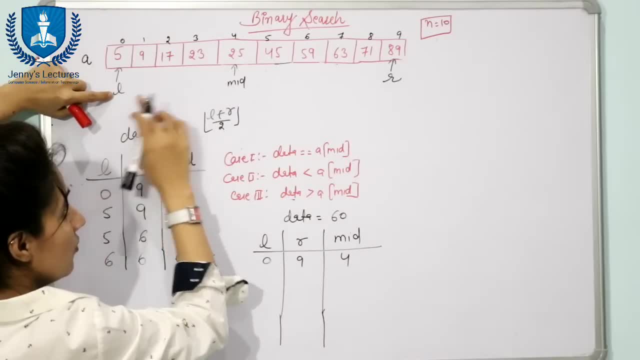 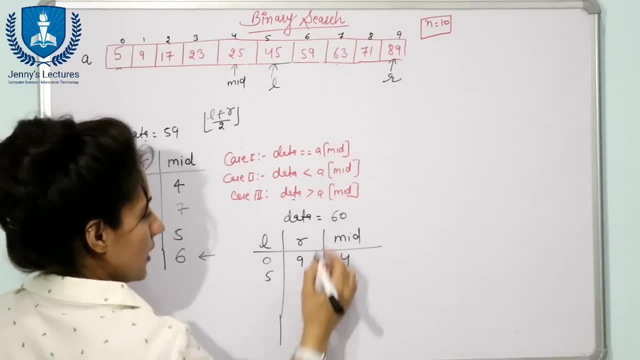 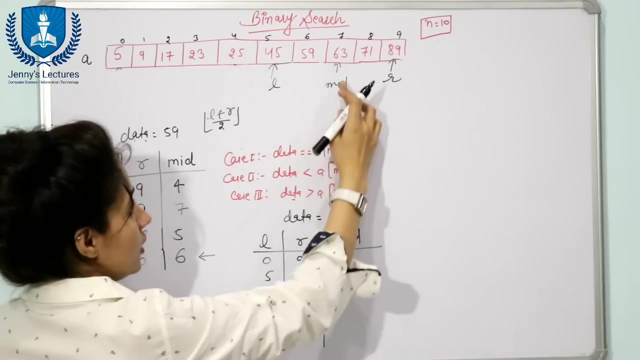 is present to the right of this one, then we are going to move this left and left becomes mid plus 1 here. now left is 4 plus 1 is 5 and right remains as it is. again, find out the middle element. that is 7. now mid is at here. only now check data: is 60, is 60, is equal to 63, a of mid? no, first case, no that. 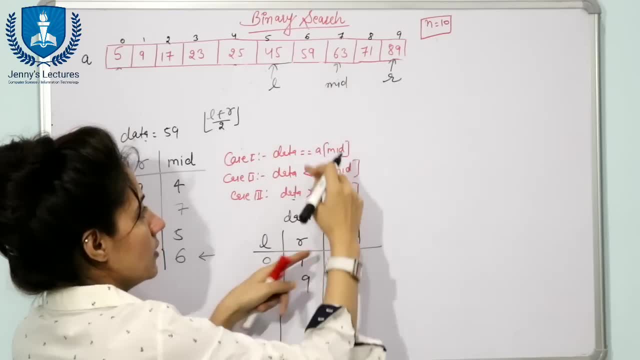 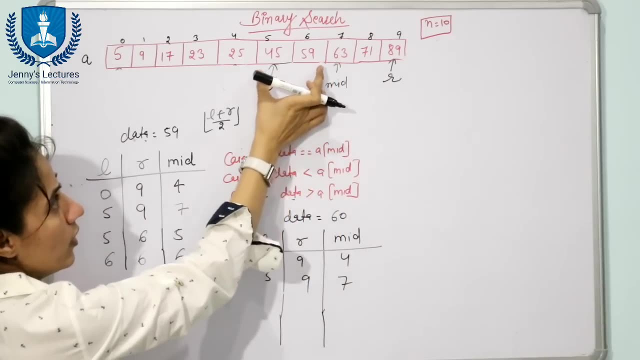 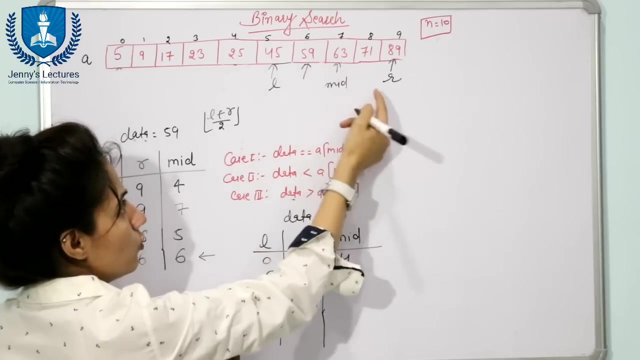 is not true. data is less than a of mid. second case is true if less than it means the data is present to the left of left of 63. then we are going to work in this array: left becomes as it is in that case. in that case, right becomes mid minus 1. so here we are going to shift this right. 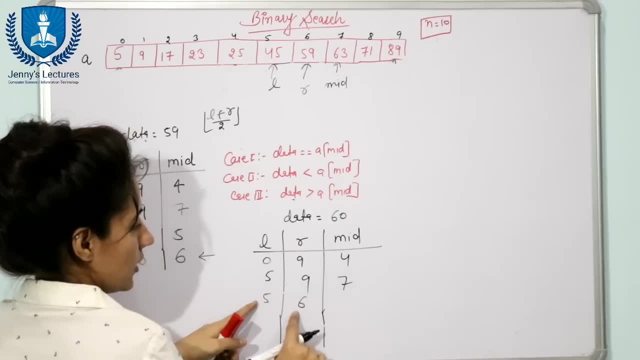 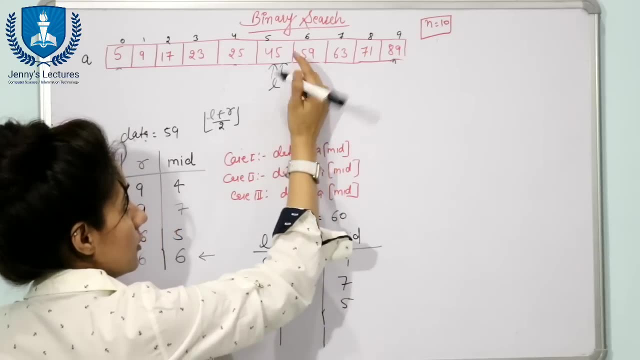 now right becomes mid minus 1, that is 6. again the middle element, that is 5. so now mid is at 5. right here, all here we have mid. now check if data is equal to mid. 60 is equal to 45, no, 60 is. 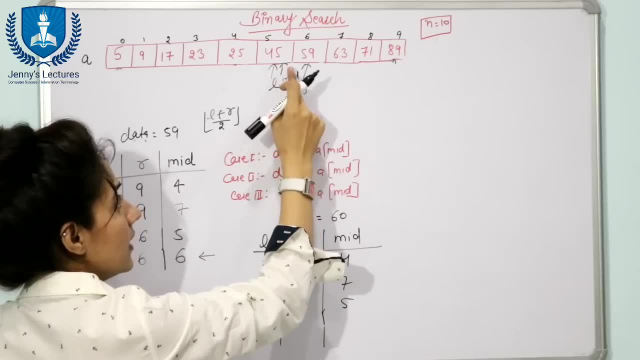 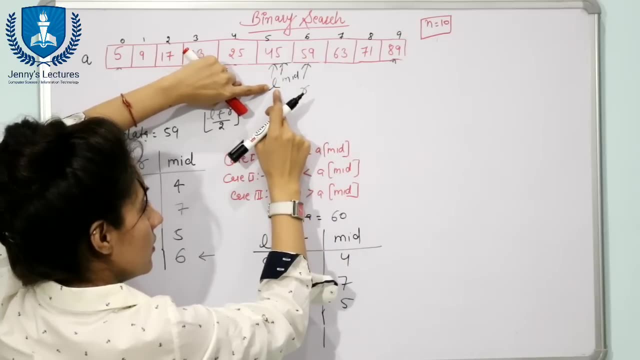 greater than mid. this condition is true if greater than, if greater than then data was would be to the right of this right of mid. so in that case, we are going to shift this right now. right becomes mid plus 1, and we are going to move this left to this side. so, left, this l becomes now mid plus 1, that is. 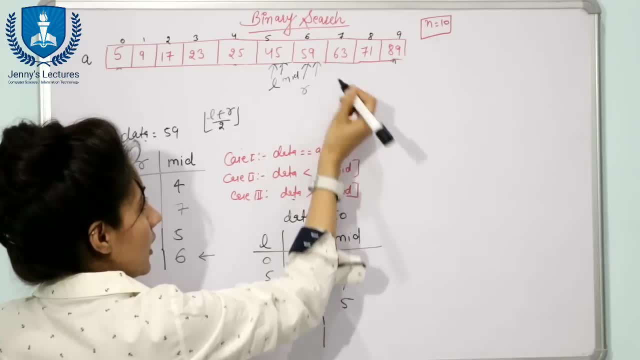 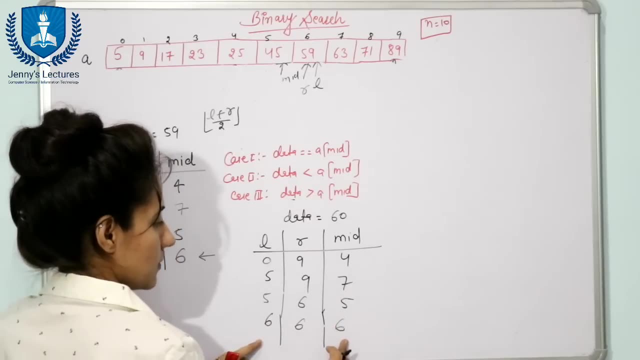 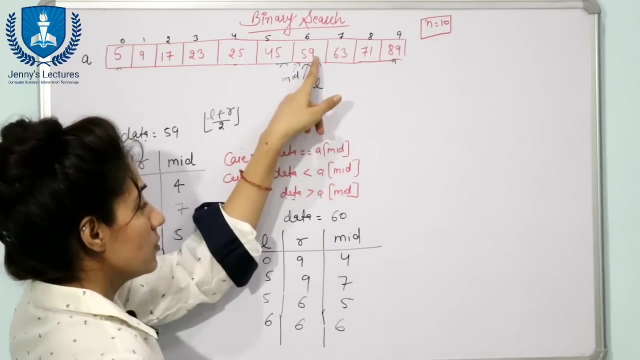 6 and right remains as it is. so now, here we have what left and right both now middle element is 6, now middle 6 now here also we have mid. now check this data: 60 is equal to this mid. no, this 60 is what greater than this data it means. 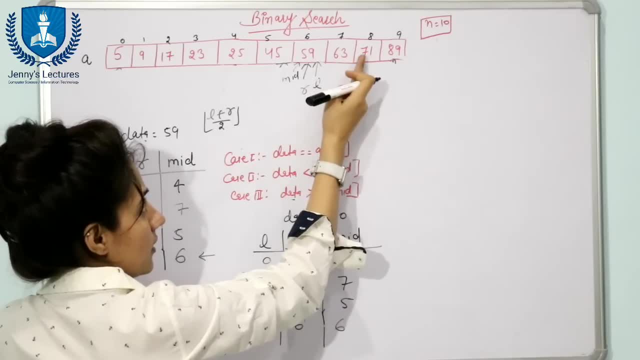 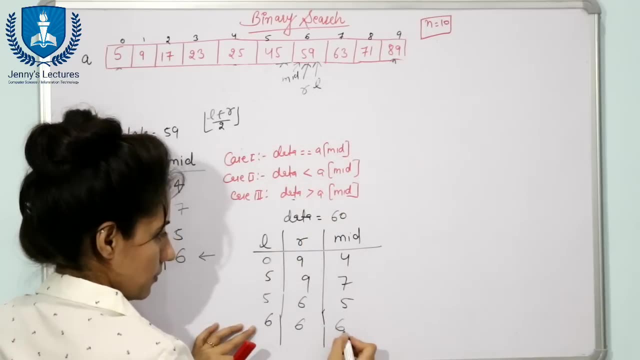 the data is present to the right of this 59 right, and if data is present to the right array, then we are going to move this l. l becomes mid plus 1 now, l becomes 6 plus 1 is 7 and r remains as it is now. 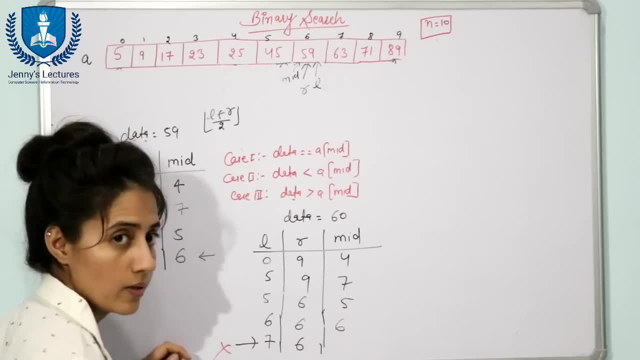 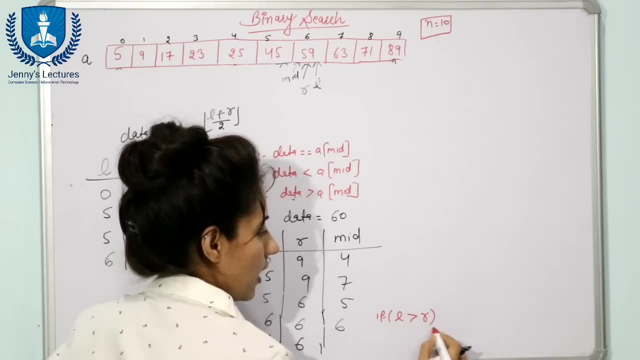 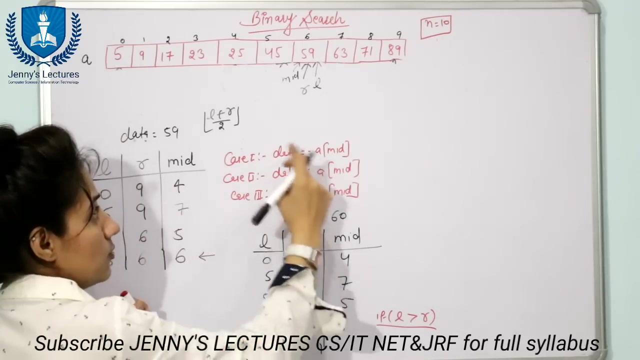 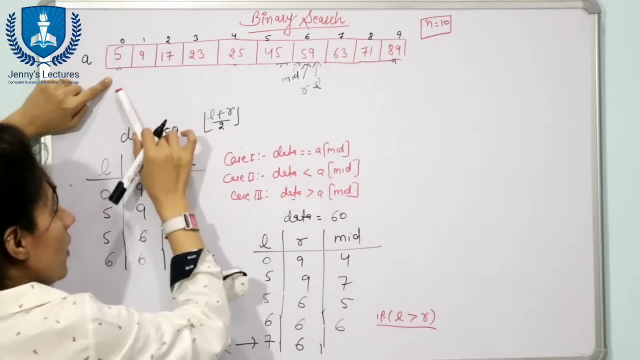 this is the stopping condition here. if this l value, if l value becomes greater than r value, it means data is not present. here we are going to repeat these steps. find out the mid. checking these conditions till l is less than right, because here we have taken left, here we have taken right. once this left becomes, 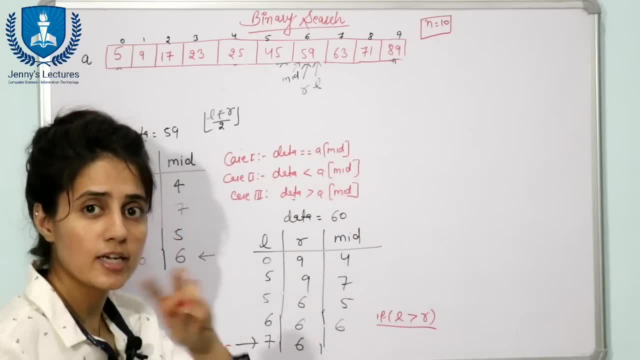 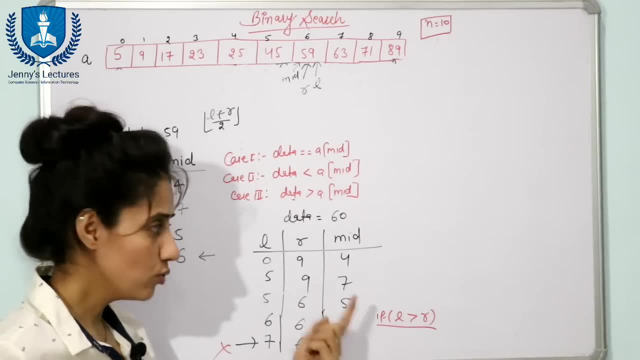 greater than right. they have crossed each other. it means data is not present, so this is the stopping condition. in that case, if data is not present right now, i am going to write a piece of code for this binary search. see, i am going to create a function: binary search. 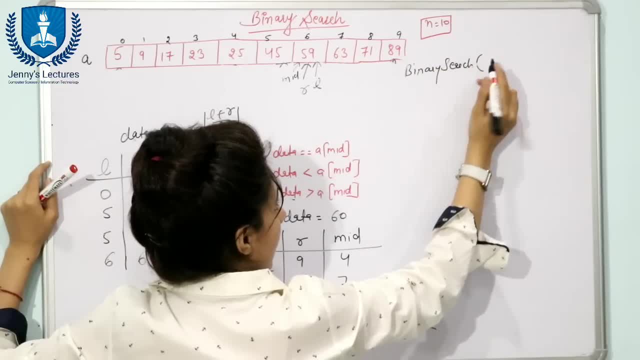 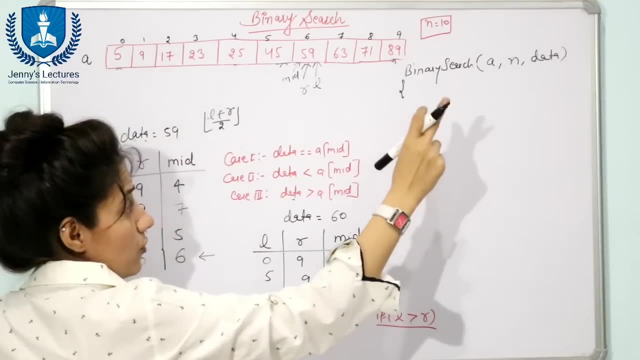 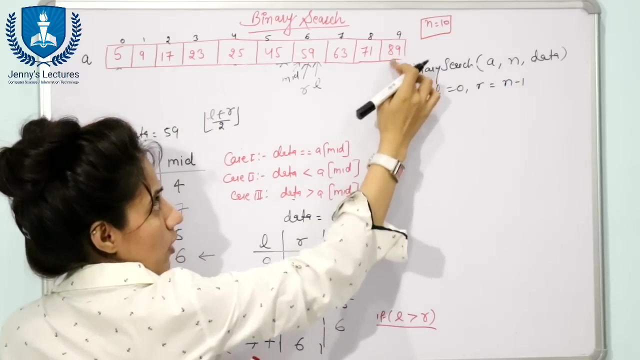 in this i am going to pass array, a total number of elements in the array and the data you want to search. so now, first of all, what we have done. we have taken: l is equal to 0 and r is equal to n minus 1. n is 10, so r was 9, fine, and after that we have calculated what mid. so now, 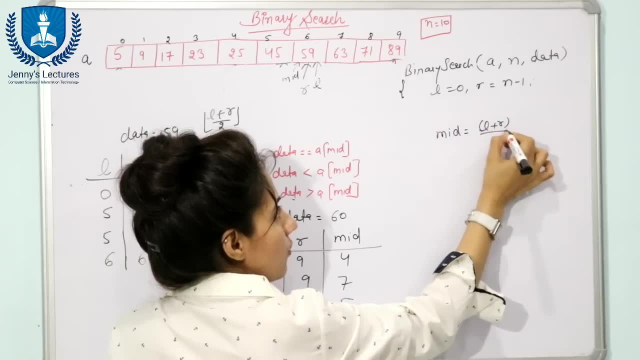 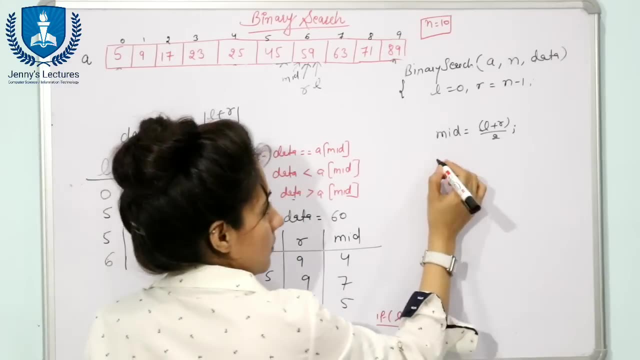 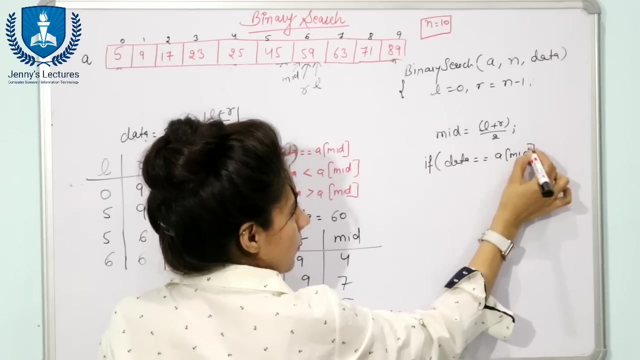 mid is equal to l plus r divided by a 2. right after calculating mid, we are checked. three conditions right, three cases can be there. so we have checked if data is equal to is equal to a of mid. if this is true, then you will do what? 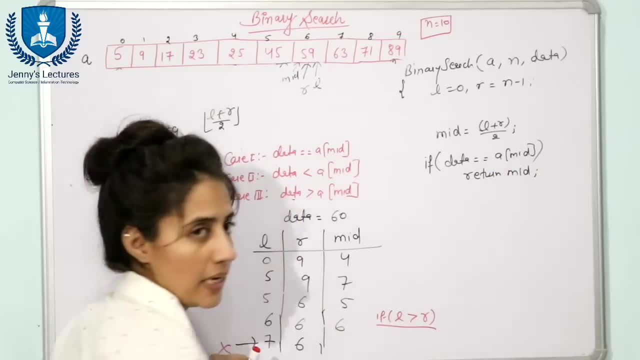 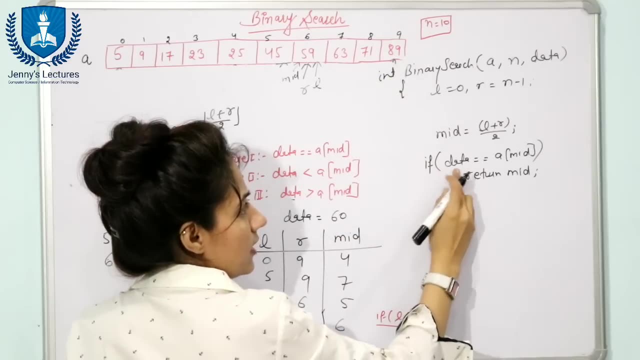 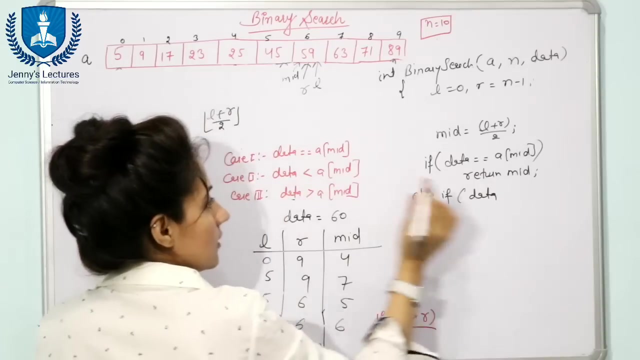 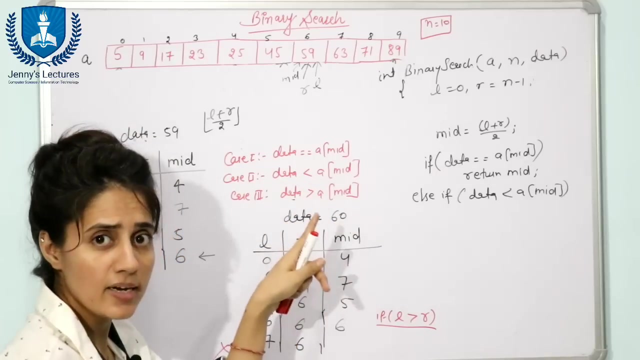 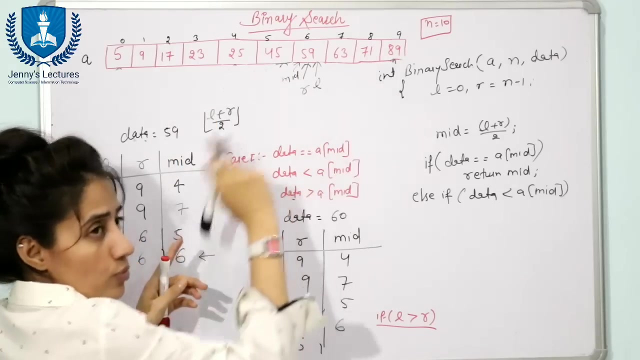 return mid. here you are returning some integer value, so the data type would be int, right, if this condition is not true. else, if data is less than a of mid, if data is less than a of mid, less than a of mid, less than means data is present to the left side of this mid, it means r value would be. 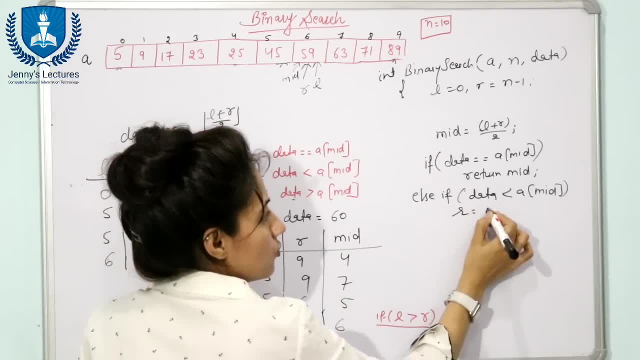 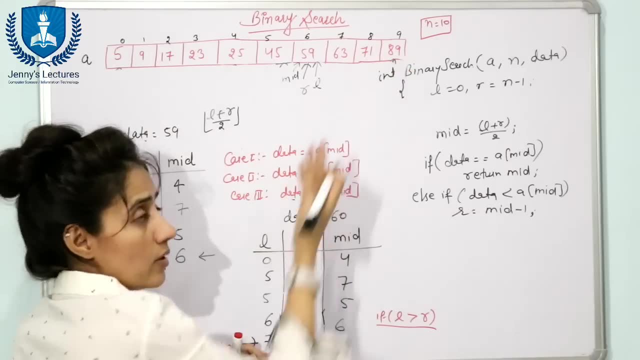 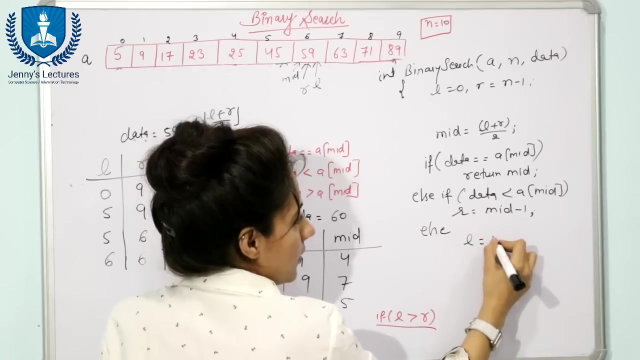 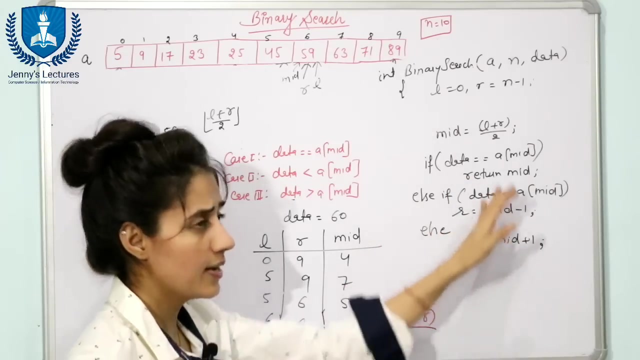 L value remains as it is. so now r becomes mid minus one right. and the third case, as data is present, to the right of the smith. in that case you will move left. left becomes mid plus 1, else l becomes mid plus 1 right, and you are going to repeat these steps till left l is. 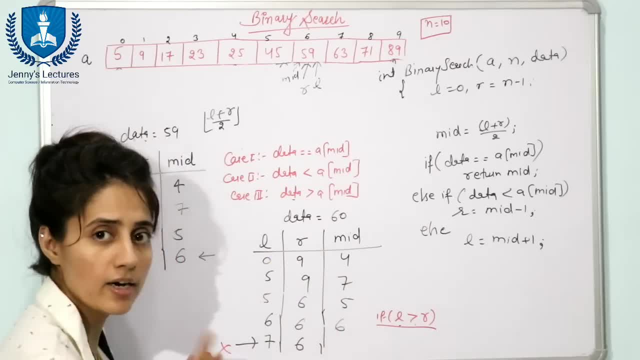 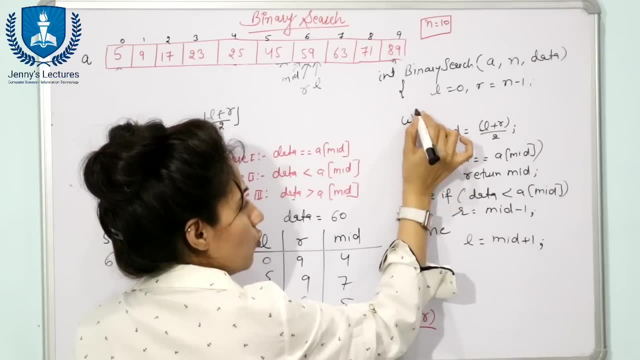 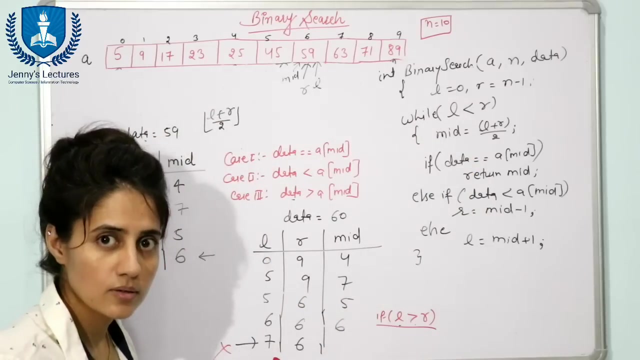 less than r. once l becomes greater than r, it means data not found right. so you are going to repeat these steps. so you are going to write down these steps in a loop, that is, while l is less than r, till then these steps should be repeated. if l is not less than r, it means obviously l would. 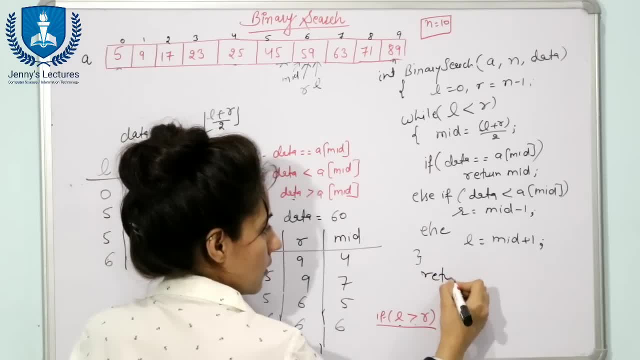 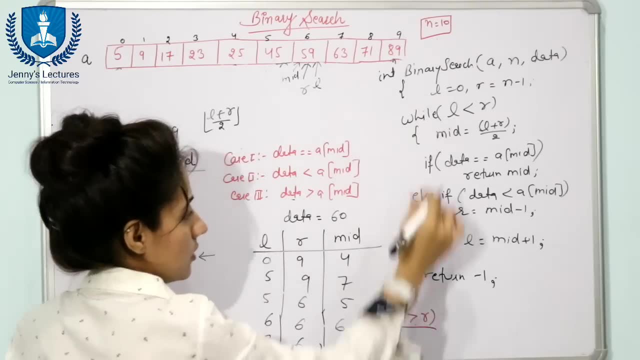 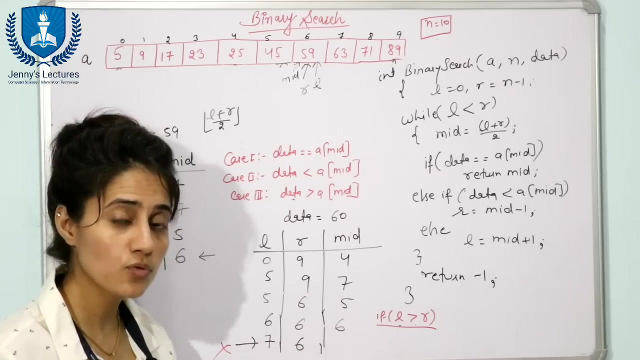 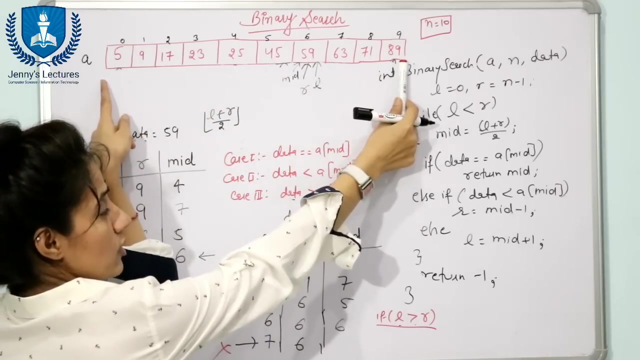 be greater than r. so here you can return what minus 1. minus 1 means. data is not present, right, and you can close this function. so this is how the binary search is going to work. now, what is the time complexity for this algorithm? see, we are. we are reducing the search space by half. at first, search space was this one, again by. 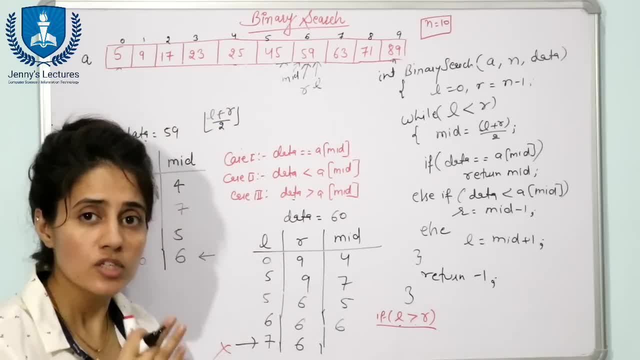 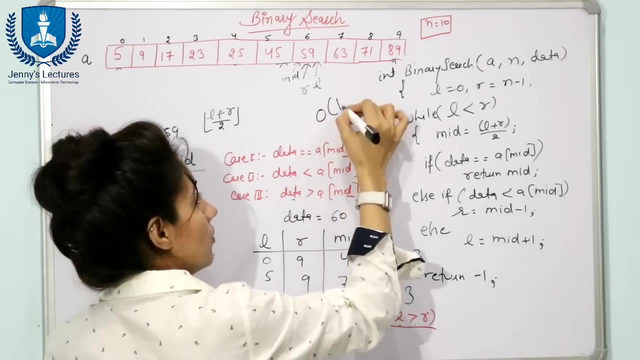 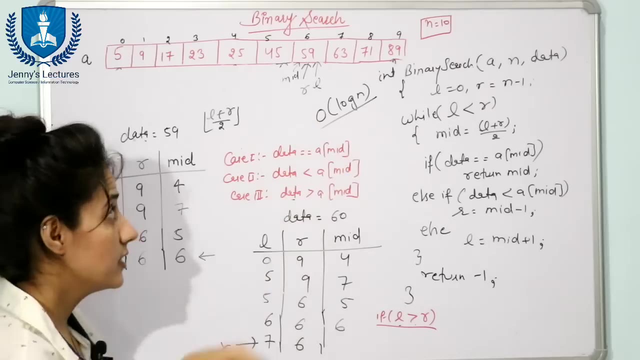 half again, by half again by half, like this. so if such kind of behavior exists, in that case time complexity would always be order of log n. in worst case it is order of log n. and what is the time complexity in best case? see, suppose i am going to find the data: 25. data is 25. 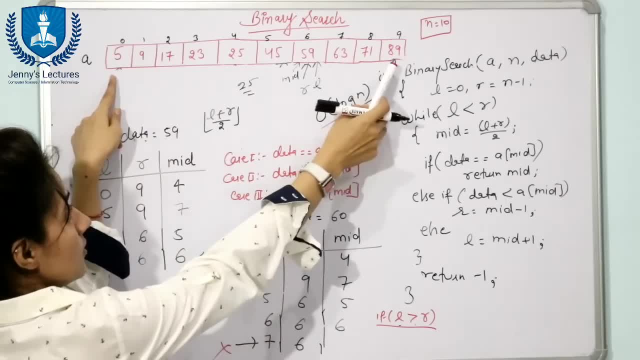 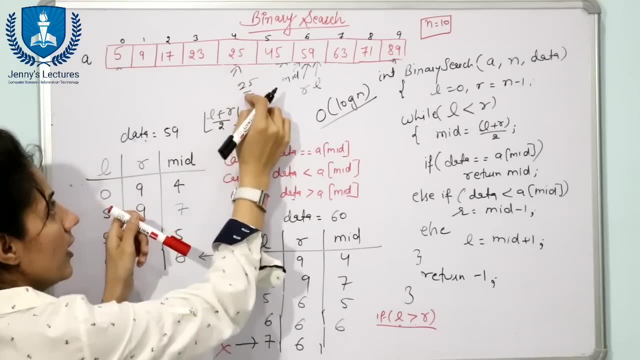 at first. i am calculating l plus 9 plus 0, divided by 2, that is 4, and at 4 is mid is at 4. now, here only i got 25. so this is what the best case, in best case, time, complexity would be. order of. 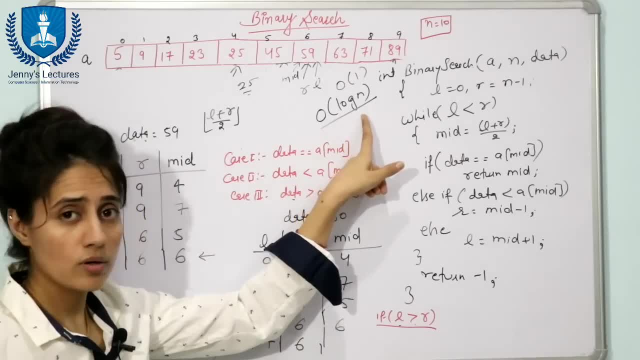 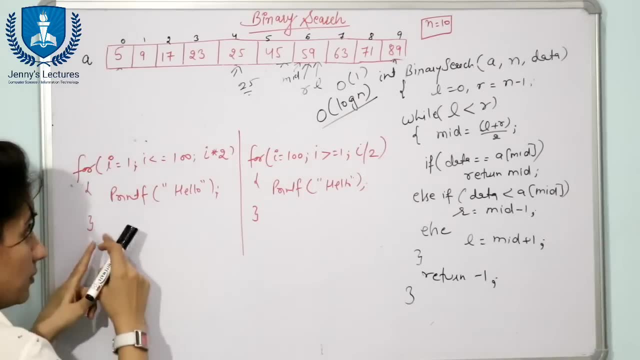 1 right and in worst case it is order of log n. see now why i am saying this order of log n. i am going to tell you with the help of an example. see, let us take these two cases. i am just going to take these two for loops, simple for. 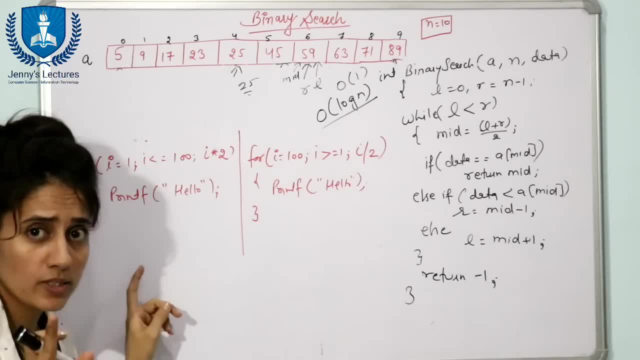 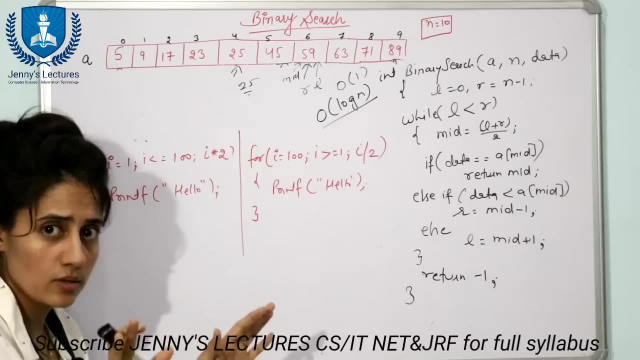 loops. i am going to calculate the time complexity for this, and this also time complexity means we are going to find out within this four loop, the statements is going to execute how many times. right, that is the time complexity now in this case. in this case, how many times? 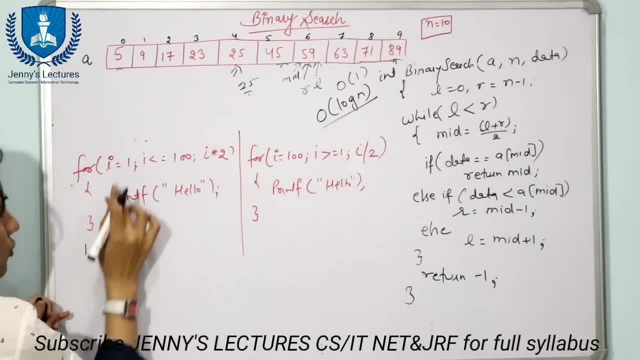 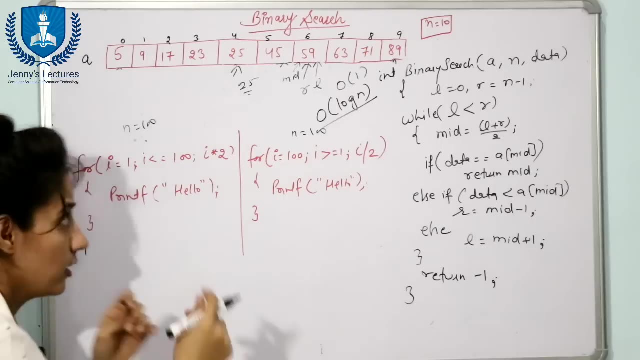 the statement within this for loop would be executed. see: i is equal to 1, i less than 100. here, n is equal to 100. here also, n is equal to 100. fine, so so this is going to be executed. now i into 2. here i am going to double the value of i. 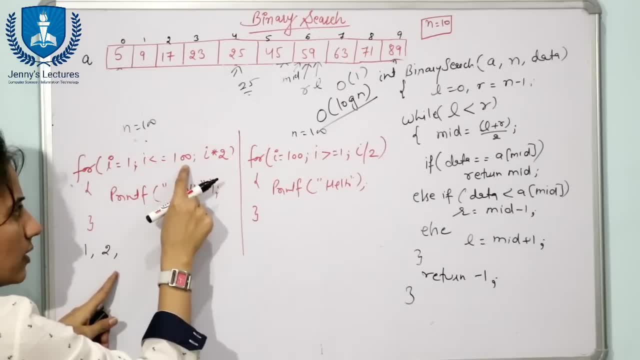 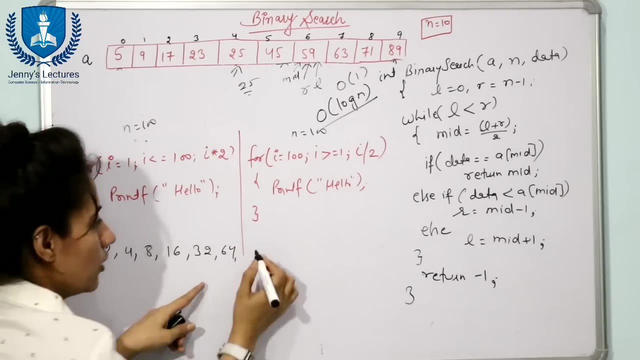 so now, next time becomes i value becomes 2: 2 is also less than 100. now again, it would be executed. now, next time it becomes 4: 4 is also less than 100. now, next time it becomes 8, next 16, 32, 64, and after that it becomes what? 128, 128 and 128 is not less than 100. 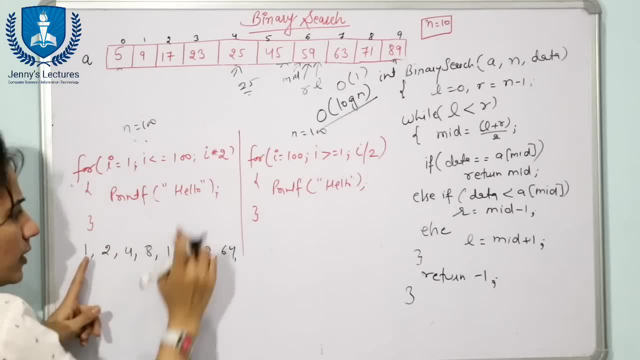 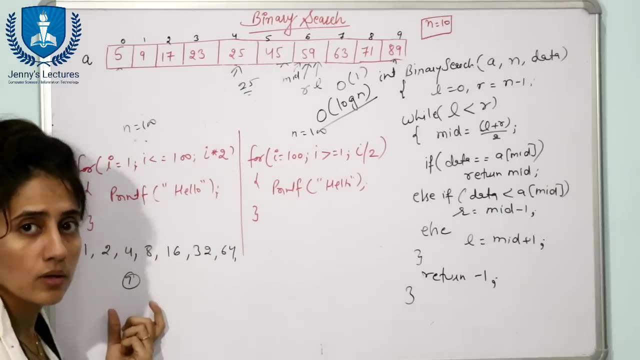 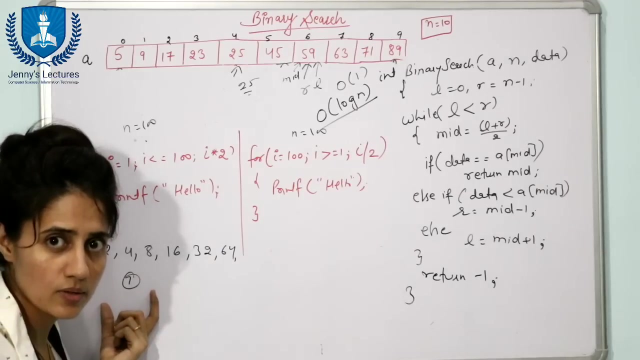 so this is not going to be executed. so how many times this statement would be executed? 1, 2, 3, 4, 5, 6, 7, 7 times and n value was 100. for the value 100, how many times the statement would be executed? only for 7 times. right same here. in this case, n value is hundred. how many? 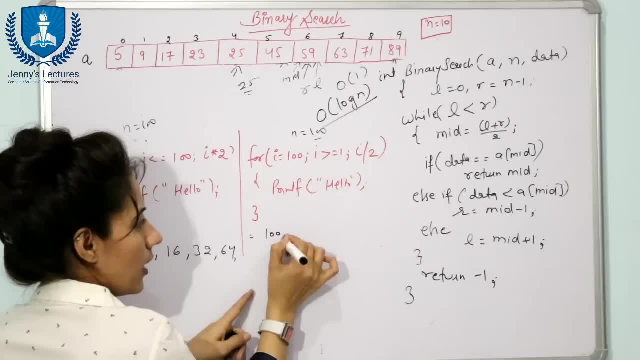 times. this should be executed at first. i is equal to 100. now i am going to divide the i value by 2, i am going to divide by 4.. okay, Okay, here you see this. i value once again. this is 10 in fact. i will be writing down. 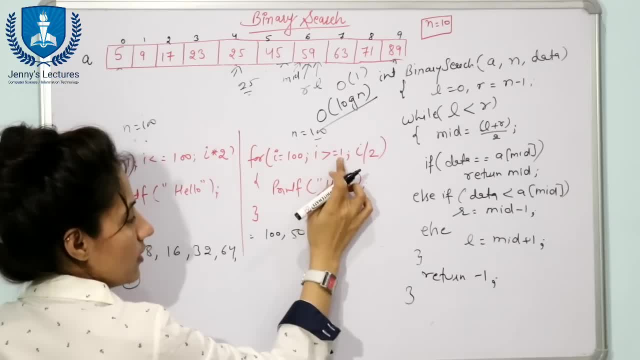 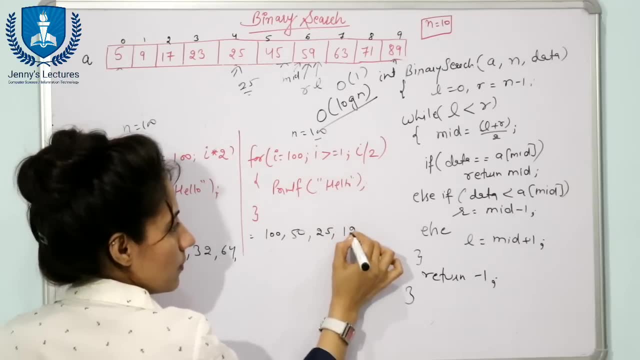 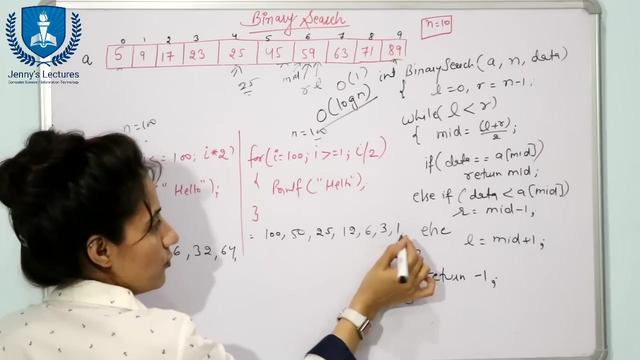 it by half next time: 50. 50 is greater than equal to 1. okay, next is 25. 25 is also. it would be executed next time. divided by 2 is 12, next time 6, next time 3, next time, 1. next time. if you divide. 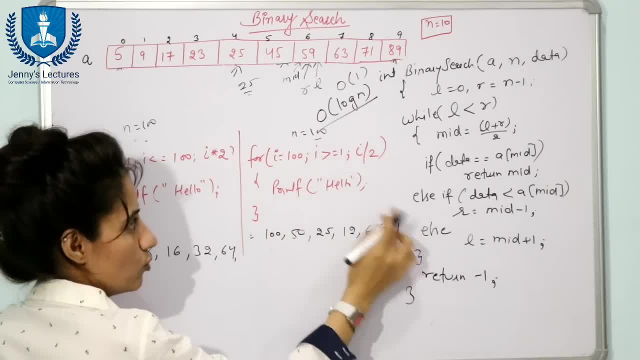 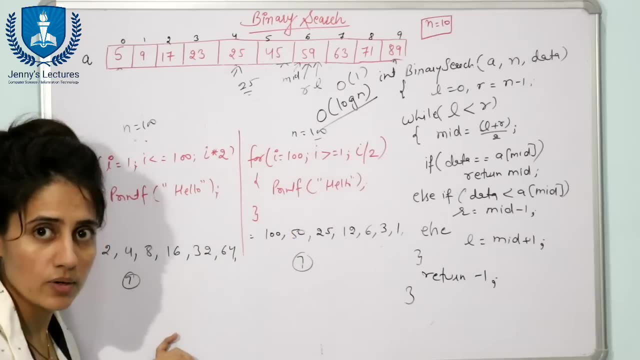 it becomes what? 0, 0 is not greater than equal to 1, so it is going to stop. it is not going to execute now. here also 7 times: 1, 2, 3, 4, 5, 6, 7, 7 times. here also: n value is 100, right. 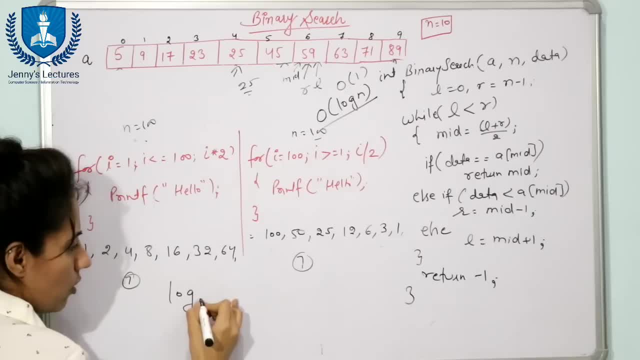 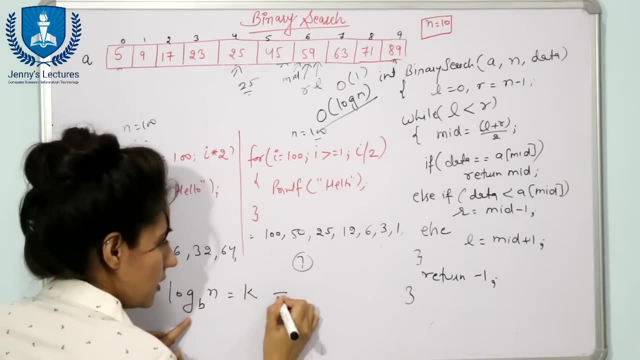 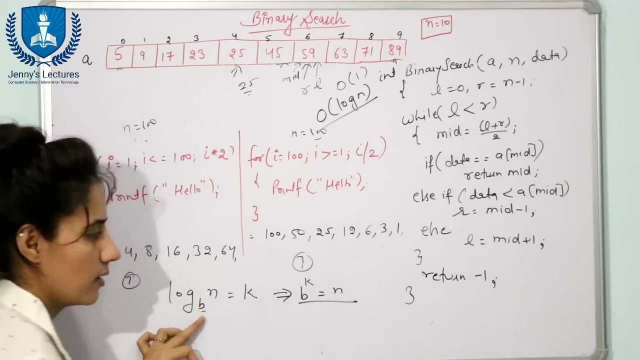 i hope you know the formula of this thing: log of base b and n is equal to k. it means it means this: b, b of b, power, k is equal to n, right? this is the formula. if this is the case, then you can say that b of k is equal to n. if you, if this is the case, b of k is equal to n. 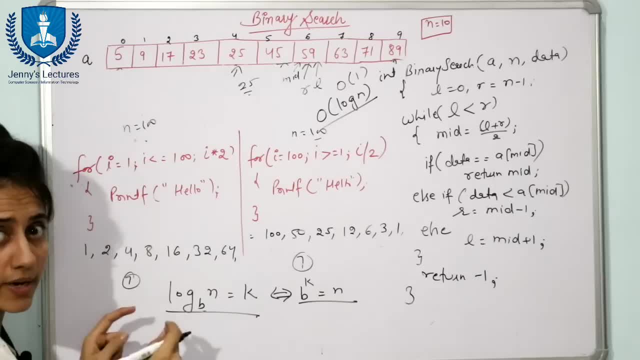 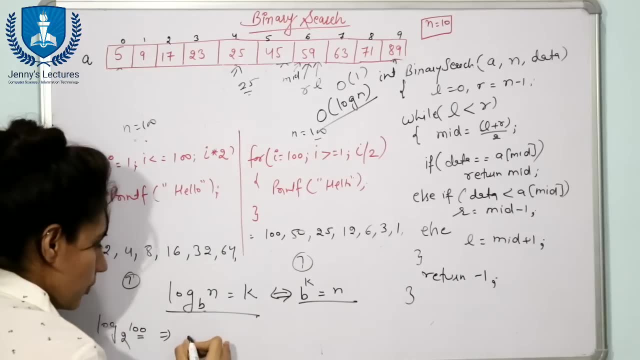 it means you can say: log of b: n is equal to k, now here n is equal to 100. now, if you put log of 2 and 100, what you can write: 2 raised to power, 2 raised to power what 7? because 2 raised to power 6 is what 64 and 64 is not. so i can write: 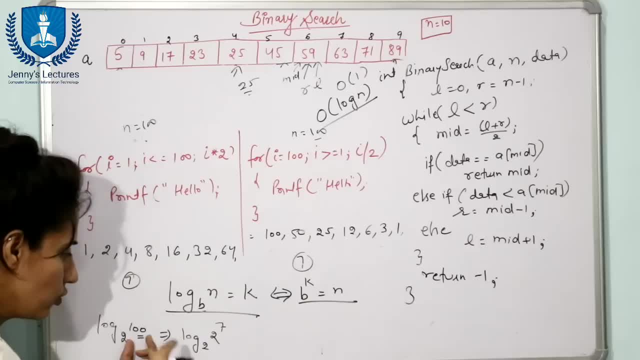 2 raised to power 7, that is 128. so i can write 7, but i cannot write 6 because 64 is less than 100 but greater than value we can write. so we can take here 2 raised to power approximately 7. so 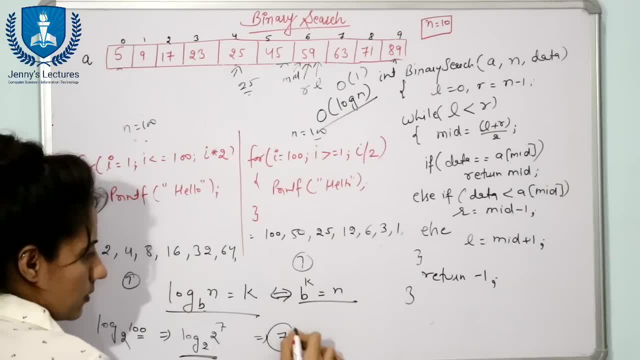 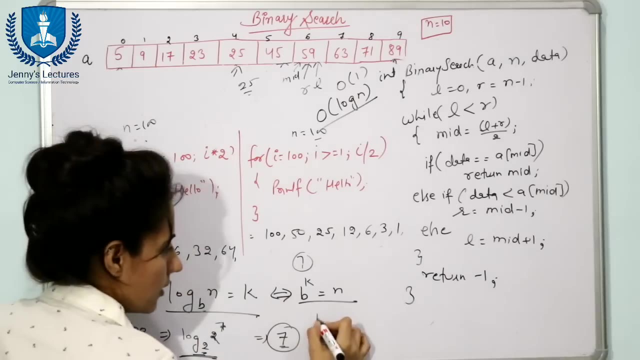 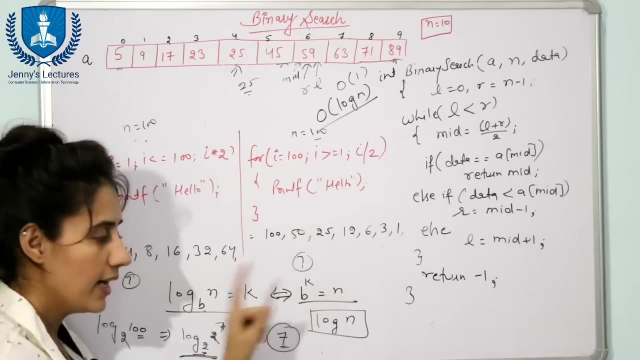 it means it becomes what 7? only right, because base is also 2 and here also 2. it means we, we just take only the power, that is 7. fine, so the time complexity, how many times this loop has been executed? log n times. right, here also you can say log n times. so if such kind of behavior occurs, if